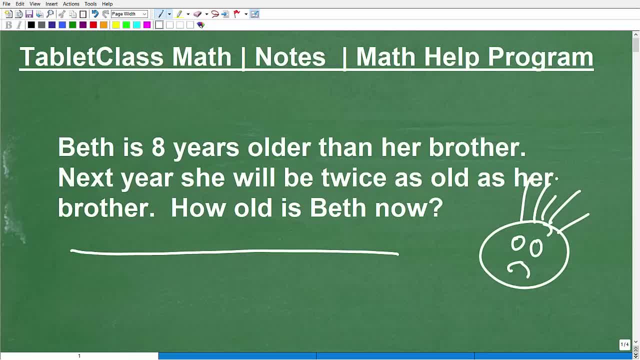 Unfortunately, in mathematics there are word problems, And word problems are an application of the skills that you are learning. But there's no reason to fear word problems. I know that they're scary and whatnot, But what we have to do is reduce that fear. And the way you reduce that fear of word problems is: one: you got to build up your skills, Okay, And then two, you have to have, you know, the basic kind of guidelines. You got to have some general guidelines on how to approach. 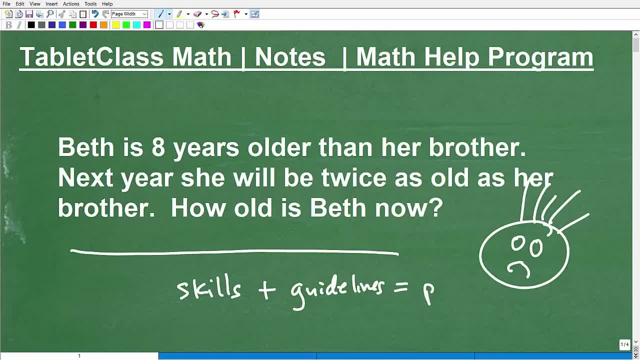 word problems. And then obviously you have to practice word problems, Okay, And if you don't practice word problems you're not going to get better at them. So we're going to take a look at this classic algebra word problem. It's an age word problem And I'm sure I did this work, this flavor of word problem, way back in the good old 1980s when I was in high school, not paying attention, not doing what I was supposed to do, But I'm sure my teacher was trying to get me to understand this stuff, And then even your, my grandparents, probably were even doing it. 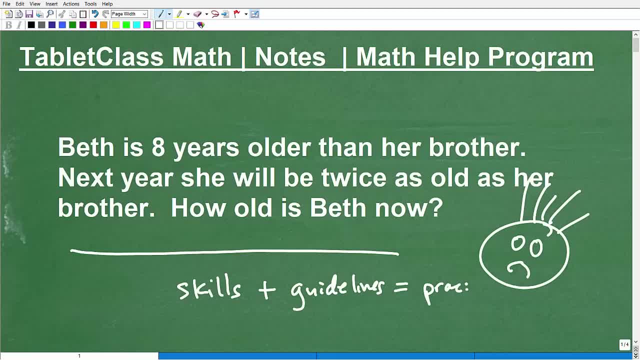 And you know this is a kind of again in algebra the word problems that you study are. you know they've been taught for years and years and years and years. So as you understand these general type of word problems- age word problems are kind of classic- then you should be pretty good to go on your test. So no need to be afraid We're going to erase this guy here, But let's get into how we approach a word problem And then obviously I'm going to solve this word problem. 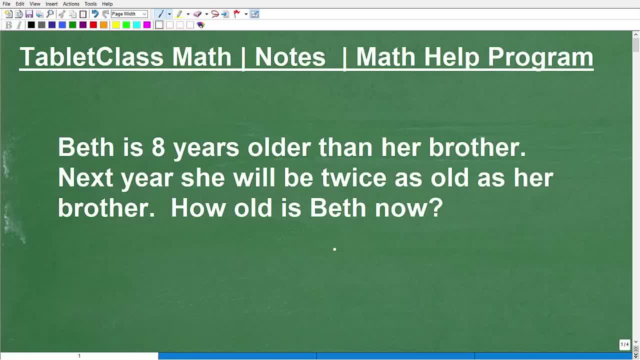 Here in a second, So I'm going to talk about all of this in just one second, But first let me quickly introduce myself. My name is John. I'm the founder of Tablet Class Math. I'm also a middle and high school math teacher And over several years I've constructed what I like to believe. What I like to believe is one of the best online math help programs there is. That's a pretty bold statement, But I really, truly believe I have created an awesome program. Of course, I'll let you be the judge of that. If you're interested, you can find a link to my math help program in the description of this video. 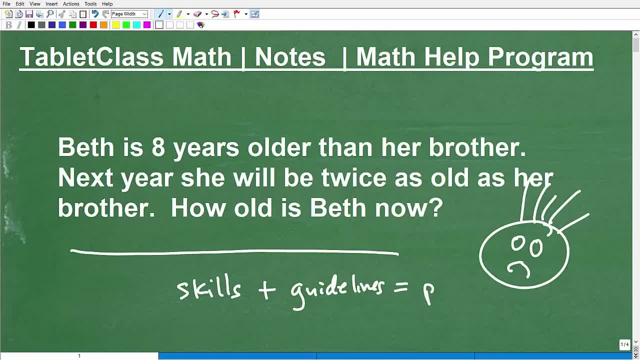 word problems. And then obviously you have to practice word problems, Okay, And if you don't practice word problems you're not going to get better at them. So we're going to take a look at this classic algebra word problem. It's an age word problem And I'm sure I did this work, this flavor of word problem, way back in the good old 1980s when I was in high school, not paying attention, not doing what I was supposed to do, But I'm sure my teacher was trying to get me to understand this stuff, And then even your, my grandparents, probably were even doing it. 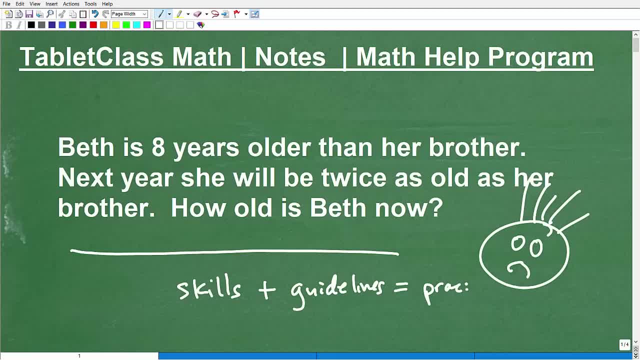 And you know this is a kind of again in algebra the word problems that you study are. you know they've been taught for years and years and years and years. So as you understand these general type of word problems- age word problems are kind of classic- then you should be pretty good to go on your test. So no need to be afraid We're going to erase this guy here, But let's get into how we approach a word problem And then obviously I'm going to solve this word problem. 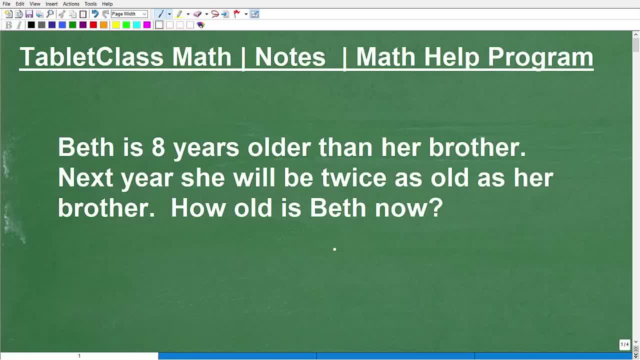 Here in a second, So I'm going to talk about all of this in just one second, But first let me quickly introduce myself. My name is John. I'm the founder of Tablet Class Math. I'm also a middle and high school math teacher And over several years I've constructed what I like to believe. What I like to believe is one of the best online math help programs there is. That's a pretty bold statement, But I really, truly believe I have created an awesome program. Of course, I'll let you be the judge of that. If you're interested, you can find a link to my math help program in the description of this video. 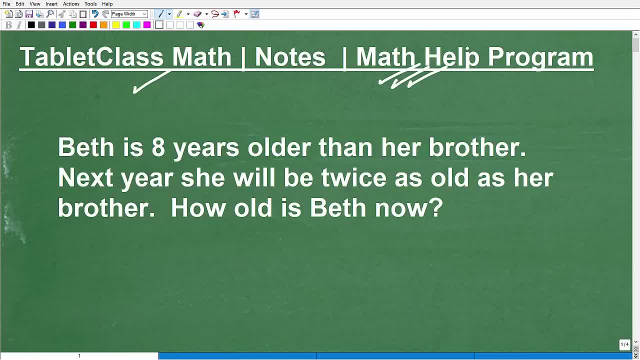 But basically I have 100 plus different math courses. I have all the main courses that people take in middle and high school, like pre-algebra, algebra 1, geometry, algebra 2. I'm going to be launching pre-calculus here soon. I also have, like college, algebra. I have all those kind of main courses, But I have many, many, many specialty courses, a lot in test preparations. So for those of you that are studying for the GED, SAT, ACT, GRE, GMAT, teacher certification, nursing entrance exam, ASVAB, you know. 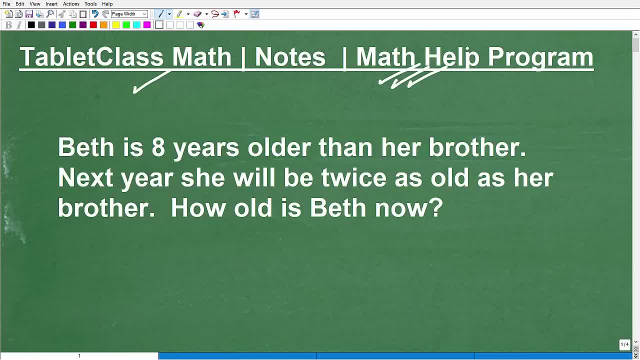 But basically I have 100 plus different math courses. I have all the main courses that people take in middle and high school, like pre-algebra, algebra 1, geometry, algebra 2. I'm going to be launching pre-calculus here soon. I also have, like college, algebra. I have all those kind of main courses, But I have many, many, many specialty courses, a lot in test preparations. So for those of you that are studying for the GED, SAT, ACT, GRE, GMAT, teacher certification, nursing entrance exam, ASVAB, you know. 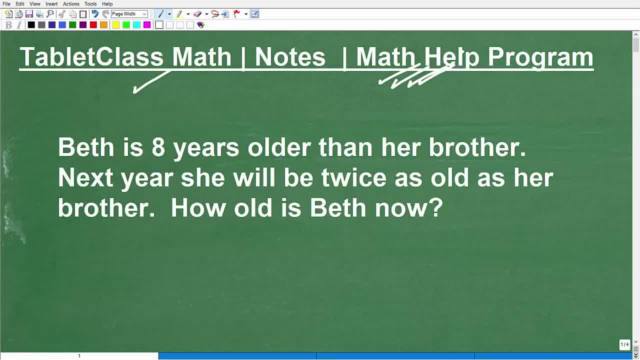 college placement, you know, end of course exams- There's a ton of really important tests that people take in their lives that a lot are, you know, a lot's written on it. Let's take, for example, a teacher certification exam. There's a lot of math on it. If you don't- you know, pass that test, the math section of it, you don't get your certification. You can't be employed as a teacher. So you know there's a lot of reasons why people study math that are outside of a math course. So I recognize that I have excellent test preparation. 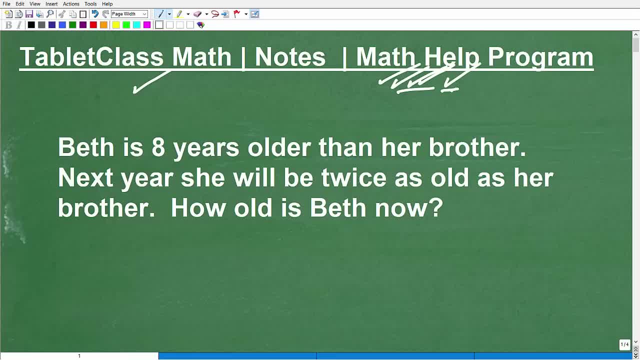 I also do a lot with independent learners, like homeschoolers. They have a great homeschool learning system. So if you are homeschooling, I can certainly help you out. And then, obviously, for those of you who are struggling in your course- let's say, you're taking algebra and you just need additional help- I can definitely help you out as well. Now, the one thing you need to be doing to help yourself out is taking great math notes. Okay, this is my golden rule of math over decades of teaching. The topic is those students who take great math notes. 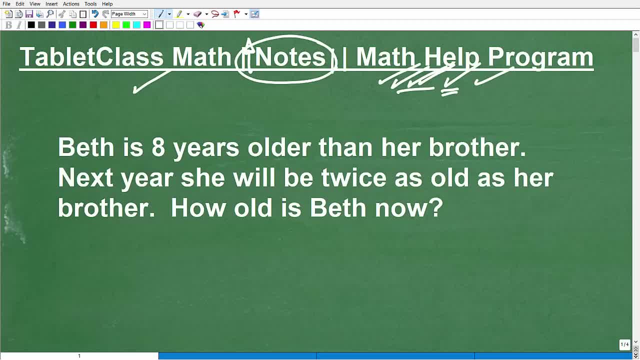 Almost always end up with excellent math grades, And the reverse is true: Those students who don't take math notes. maybe they're just like not into them. You know math notes- they're not cool, You know like, yeah, they're not necessary, because I could just listen to the teacher check in from time to time. I got a photographic memory And, plus, my best buddy in the back of the class has better notes than I, So I just go ahead and just look at their notes. Listen, that's not going to work. Okay, I'm telling you right now: you have to remain focused and engaged when you're teaching. 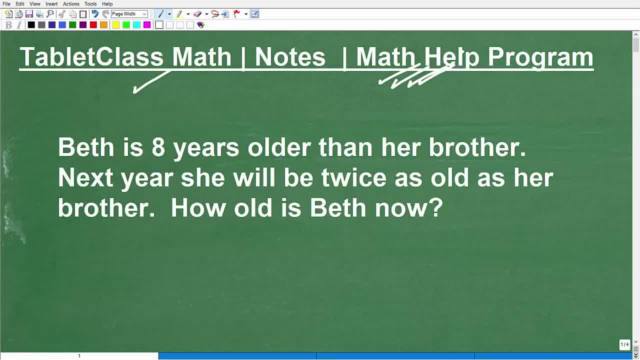 college placement, you know, end of course exams- There's a ton of really important tests that people take in their lives that a lot are, you know, a lot's written on it. Let's take, for example, a teacher certification exam. There's a lot of math on it. If you don't- you know, pass that test, the math section of it, you don't get your certification. You can't be employed as a teacher. So you know there's a lot of reasons why people study math that are outside of a math course. So I recognize that I have excellent test preparation. 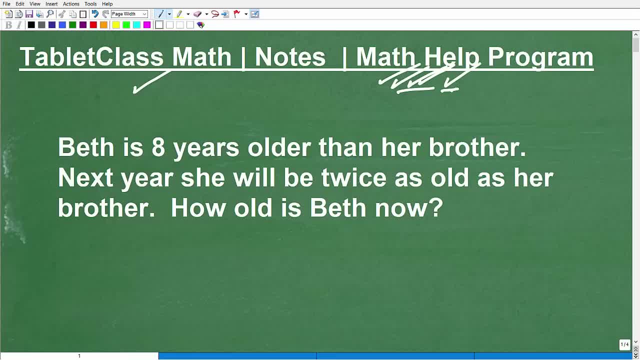 I also do a lot with independent learners, like homeschoolers. They have a great homeschool learning system. So if you are homeschooling, I can certainly help you out. And then, obviously, for those of you who are struggling in your course- let's say, you're taking algebra and you just need additional help- I can definitely help you out as well. Now, the one thing you need to be doing to help yourself out is taking great math notes. Okay, this is my golden rule of math over decades of teaching. The topic is those students who take great math notes. 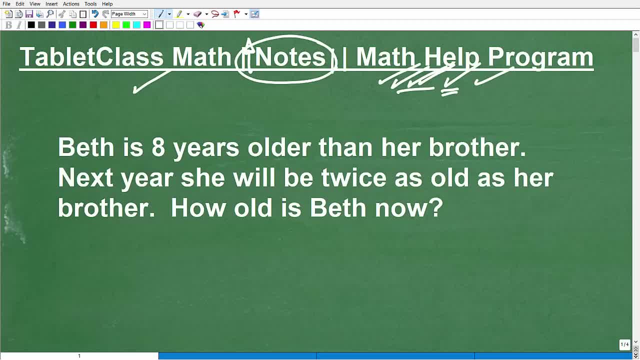 Almost always end up with excellent math grades, And the reverse is true: Those students who don't take math notes. maybe they're just like not into them. You know math notes- they're not cool, You know like, yeah, they're not necessary, because I could just listen to the teacher check in from time to time. I got a photographic memory And, plus, my best buddy in the back of the class has better notes than I, So I just go ahead and just look at their notes. Listen, that's not going to work. Okay, I'm telling you right now: you have to remain focused and engaged when you're teaching. 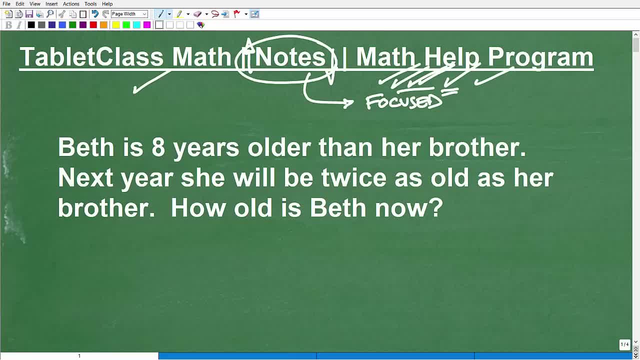 When the teacher is teaching math, Okay, that's. even if you're learning online doesn't make a difference. If you're distracted, you're not going to learn. Now, you know, I was a student once And I know what it's like to be distracted because I was distracted. But if you're going to learn math, there's only one way to really learn it, And that is to remain engaged and focused. If not, you're going to be doing this up and down business. You know, sometimes you're learning, sometimes you're not, And this is just going to lead to a unhappy situation at the end of the year. 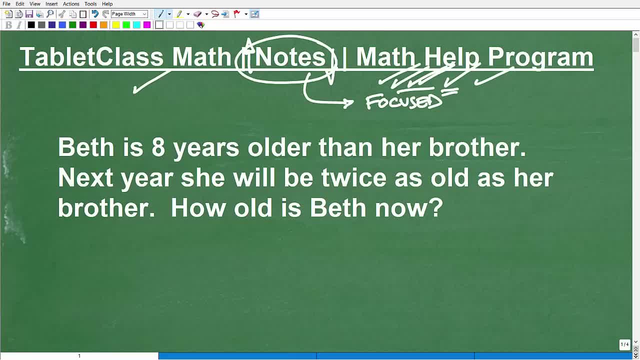 When the teacher is teaching math, Okay, that's. even if you're learning online doesn't make a difference. If you're distracted, you're not going to learn. Now, you know, I was a student once And I know what it's like to be distracted because I was distracted. But if you're going to learn math, there's only one way to really learn it, And that is to remain engaged and focused. If not, you're going to be doing this up and down business. You know, sometimes you're learning, sometimes you're not, And this is just going to lead to a unhappy situation at the end of the year. 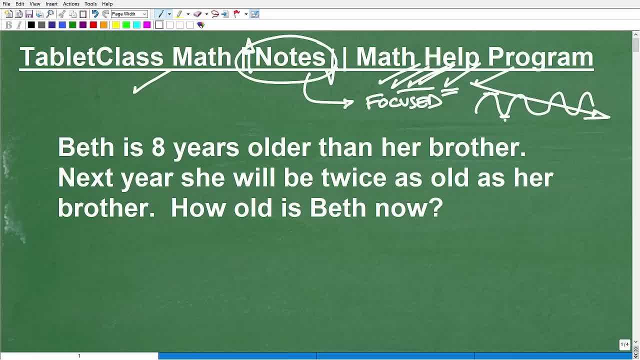 Okay, because math builds upon itself. You can't be learning math sometimes And oh yeah, you know not, And I, it's work to stay focused. Okay, so your note taking is evidence that you are remaining focused, etc. etc. So improve in your note taking. Most of you need to do this Now. in the meantime, you need something to study from, So I offer detailed, comprehensive math notes to include pre algebra, algebra one, geometry, algebra two and trigonometry. Find links to those notes in the description of this video. Okay, so here is 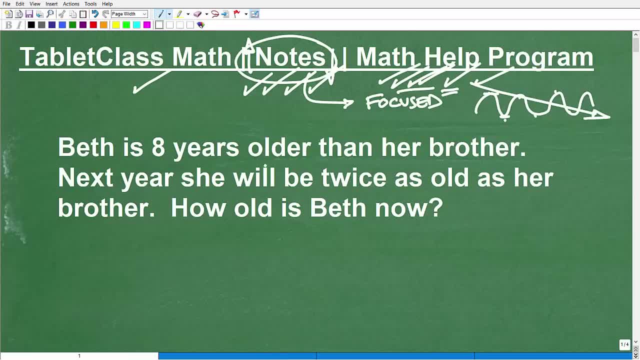 our word problem. Let's go ahead and read it real quick. Beth is eight years older than her brother. Next year she'll be twice as old as her brother. How old is Beth now? Okay, so how do we approach a word problem? Well, first thing we need to do is read it. Now. a lot of you are out there saying, Okay, Mr YouTube guy, you know, I didn't watch your video, just to you know. have you tell me to read the problem? But no, I'm telling you right now. most students read the problem one time and then 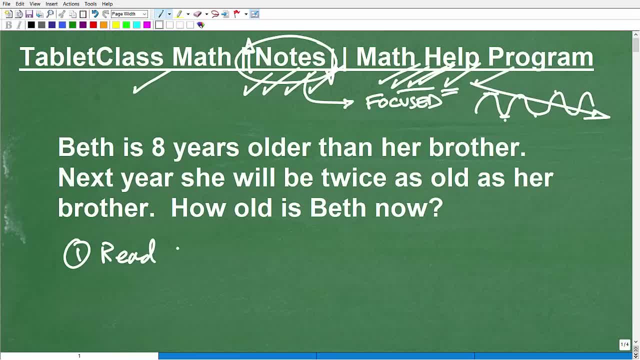 they just start working on the problem. No, that's not enough. You're gonna have to read this problem- like probably four times. Okay, so the first time you read it just get a flavor of what's going on. Okay, like, all right, read the problem And then focus in on the question mark- Here's the question mark- and then back up, because now we can identify what's being asked. Okay, what's being asked of us here? How old is Beth now? Okay, so we have Beth and her brother, And the question is: how old is Beth now? 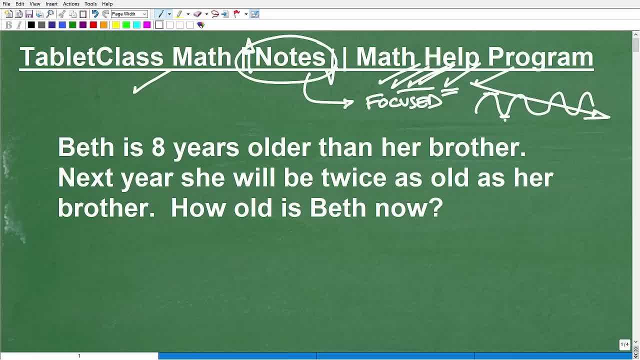 Okay, because math builds upon itself. You can't be learning math sometimes And oh yeah, you know not, And I, it's work to stay focused. Okay, so your note taking is evidence that you are remaining focused, etc. etc. So improve in your note taking. Most of you need to do this Now. in the meantime, you need something to study from, So I offer detailed, comprehensive math notes to include pre algebra, algebra one, geometry, algebra two and trigonometry. Find links to those notes in the description of this video. Okay, so here is 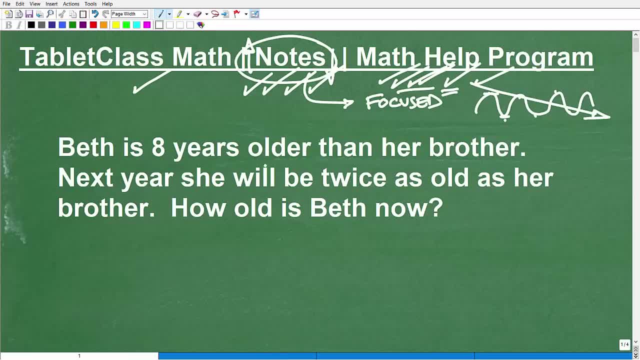 our word problem. Let's go ahead and read it real quick. Beth is eight years older than her brother. Next year she'll be twice as old as her brother. How old is Beth now? Okay, so how do we approach a word problem? Well, first thing we need to do is read it. Now. a lot of you are out there saying, Okay, Mr YouTube guy, you know, I didn't watch your video, just to you know. have you tell me to read the problem? But no, I'm telling you right now. most students read the problem one time and then 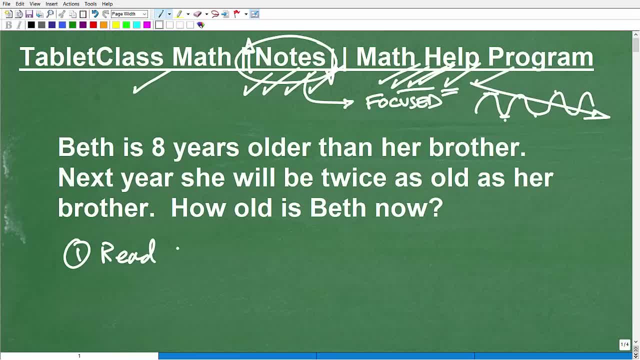 they just start working on the problem. No, that's not enough. You're gonna have to read this problem- like probably four times. Okay, so the first time you read it just get a flavor of what's going on. Okay, like, all right, read the problem And then focus in on the question mark- Here's the question mark- and then back up, because now we can identify what's being asked. Okay, what's being asked of us here? How old is Beth now? Okay, so we have Beth and her brother, And the question is: how old is Beth now? 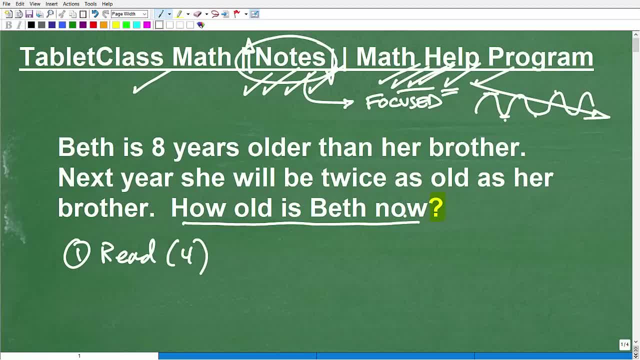 So that is what you have to focus in on, because you want to answer the specific question being asked. A lot of times, you know, students will read a problem, they'll get totally immersed, excited and they'll start doing a bunch of math and then they'll have a solution. But they forgot to answer the specific question. Okay, so we're going to read the question, get a flavor for what's being asked. Got it, Now what's the next thing we need to do? Well, oftentimes it's excellent to have some sort of 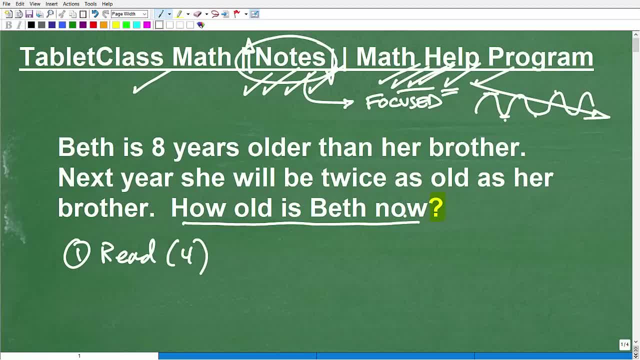 So that is what you have to focus in on, because you want to answer the specific question being asked. A lot of times, you know, students will read a problem, they'll get totally immersed, excited and they'll start doing a bunch of math and then they'll have a solution. But they forgot to answer the specific question. Okay, so we're going to read the question, get a flavor for what's being asked. Got it, Now what's the next thing we need to do? Well, oftentimes it's excellent to have some sort of 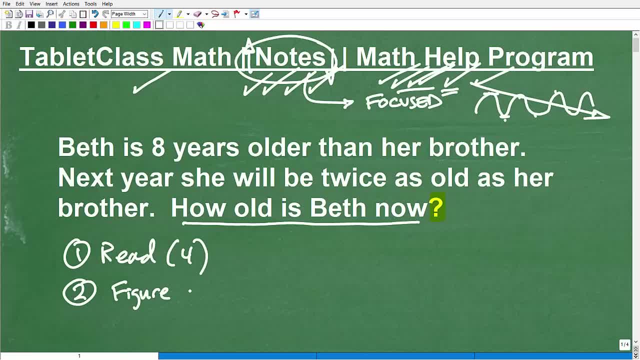 kind of sketch, right, Either a figure, if it's like a geometric situation, or some sort of model, all right, something that helps us kind of understand the situation here a little bit better. It could be like a chart, table, a graph, you know anything, but you know kind of try to put some sort of visual, you know model on what's going on, right, That's very, very useful, Okay, the next thing that we're going to want to do is establish variables. Okay, we have to assign 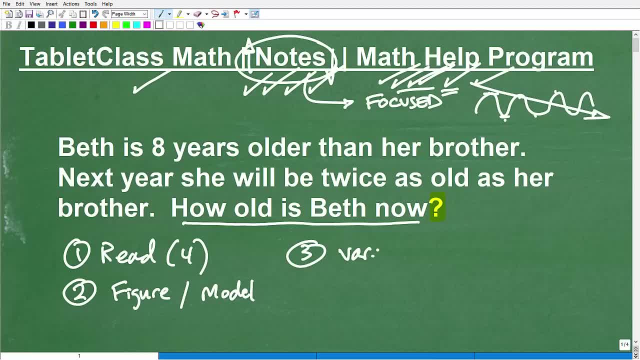 variables. So we're going to want to do is establish variables. Okay, we have to assign variables. Okay, what's being asked here? we're going to have to pick a variable like x. okay, we're going to say, okay, what's x going to be equal to? because what we're going to 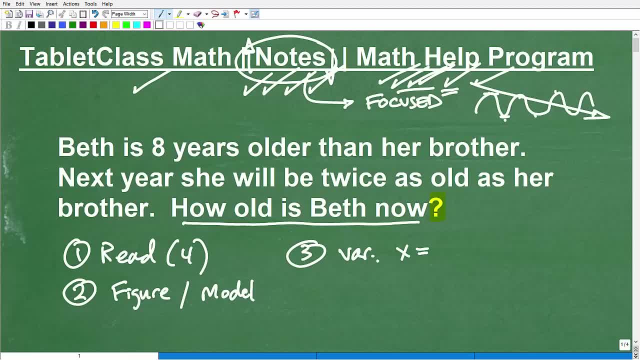 be doing here, because we are talking about algebra. we have variables. okay, we have to read this. we got this information, we have some sort of model. we're going to have to build some sort of equation. all right, some sort of equation using the information and the variables. 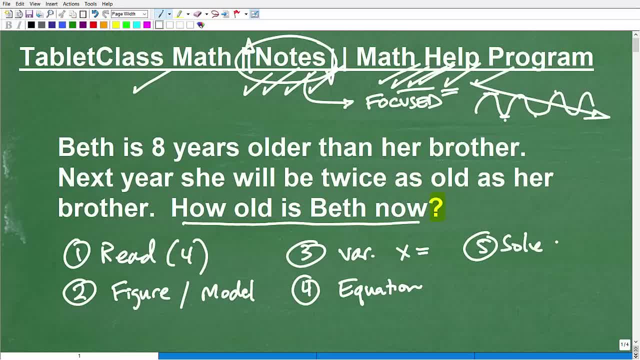 then we're going to have to solve the equation- Okay, we have to solve this equation. and then, last but not least, we're going to have to answer the right question. okay, so just because you solve the equation doesn't necessarily mean that you've answered. 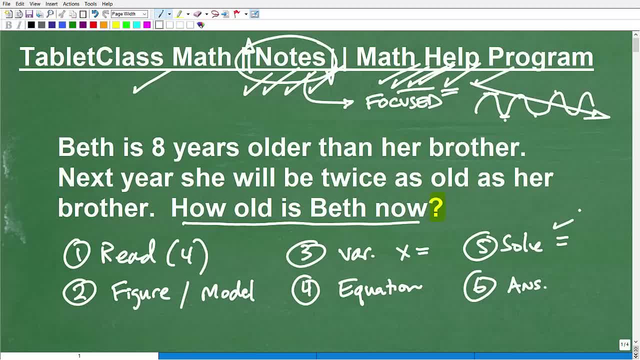 the question. okay, so we're going to see that here in this particular problem. so the only way you're going to be able to do this is to continue to read the problem, reread it and, you know, just really be fully immersed, immersed in what's going on. so this: 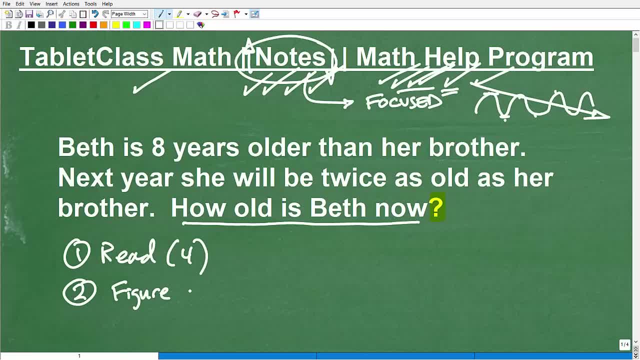 kind of sketch, right, Either a figure, if it's like a geometric situation, or some sort of model, all right, something that helps us kind of understand the situation here a little bit better. It could be like a chart, table, a graph, you know anything, but you know kind of try to put some sort of visual, you know model on what's going on, right, That's very, very useful, Okay, the next thing that we're going to want to do is establish variables. Okay, we have to assign 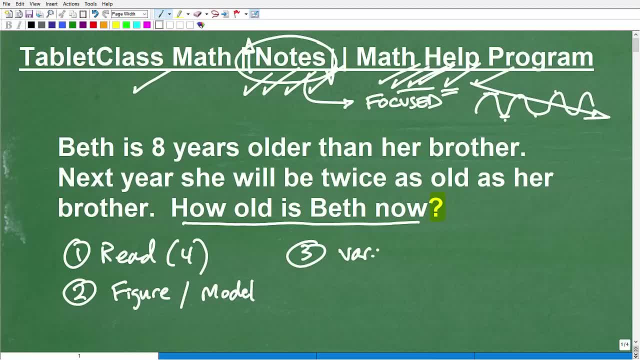 variables. So we're going to want to do is establish variables. Okay, we have to assign variables. Okay, what's being asked here? we're going to have to pick a variable like x. okay, we're going to say, okay, what's x going to be equal to? because what we're going to be doing here, because we are talking about algebra, we have variables. okay, we have to read this. we got this information, we have some sort of model. we're going to have to build some sort of equation, all right, some sort of equation using the information and the variables. then we're going to have to solve the equation. Okay, we have to. 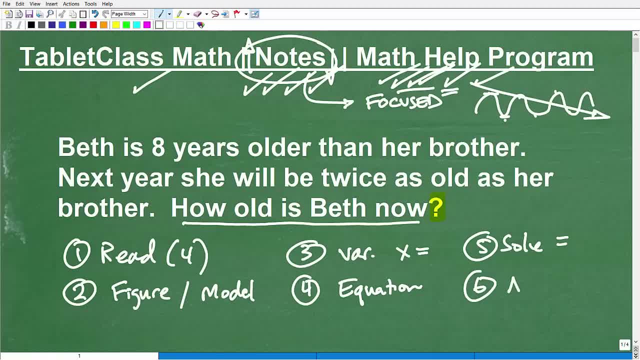 solve this equation and then, last but not least, we're going to have to answer the right question, okay? so just because you solve the equation doesn't necessarily mean that you've answered the question. okay, so we're going to see that here in this particular problem. so 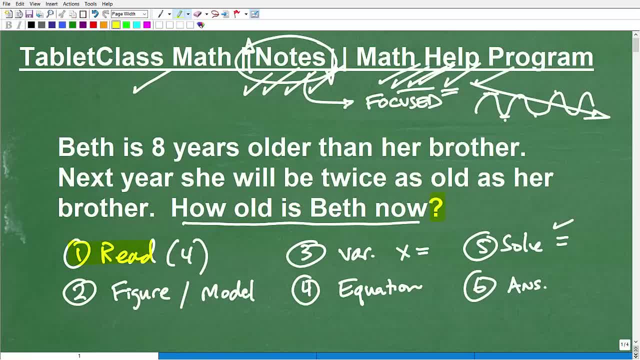 the only way you're going to be able to do this is to continue to read the problem, reread it and you know, just really be fully immersed, immersed in what's going on. so this is the kind of general guidelines to all algebra word problems and all word problems in mathematics. 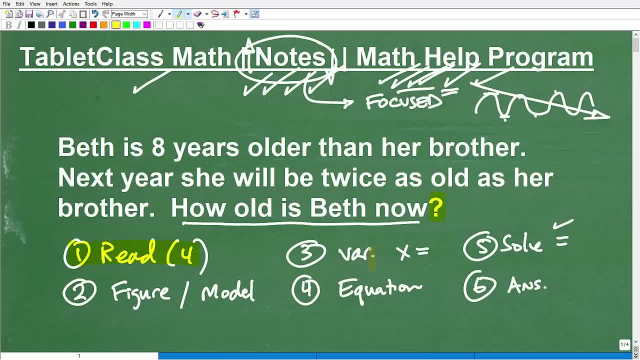 for the most part. obviously, in some courses you know, like basic math, you haven't learned yet how to solve equations, but these are kind of the general procedure or way we want to approach word problems. okay, so now, with all that being said, if you think you can do it on your own, 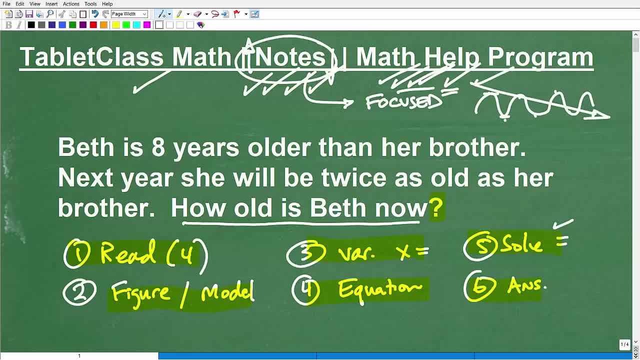 you should see. i would definitely encourage you to pause the video and try to see how you would start this problem. you don't even have to solve it perfectly. just think about it and see what you can kind of do. at least try to set up the problem, because i'm going to do it. 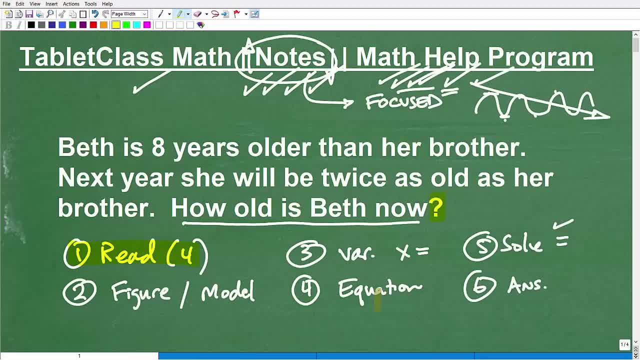 is the kind of general guidelines to all algebra word problems and all word problems in mathematics for the most part. obviously in some courses you know, like basic math, you haven't learned yet how to solve equations. but these are kind of the general procedure or way we want to approach. 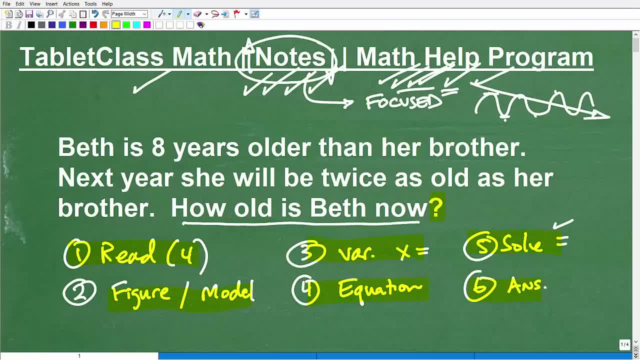 word problems. okay, so now, with all that being said, if you think you can do it on your own, you should see. i would definitely encourage you to pause the video and try to see how you would start this problem. you don't even have to solve it perfectly. just think about. 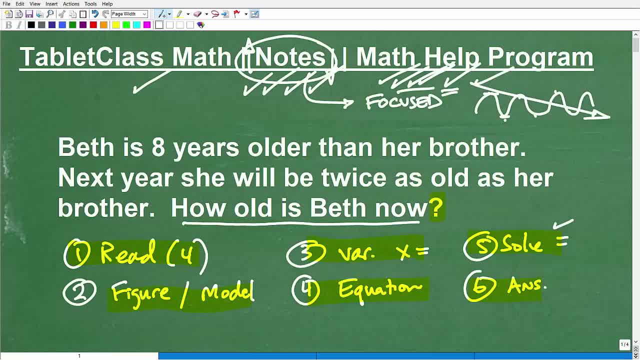 it and see what you can kind of do. at least try to set up the problem, because i'm going to do it. you're going to be like, oh, that was easy. remember, watching someone do math is not the same as learning math. okay, now i'm here to help you, obviously, but you should always try to challenge. 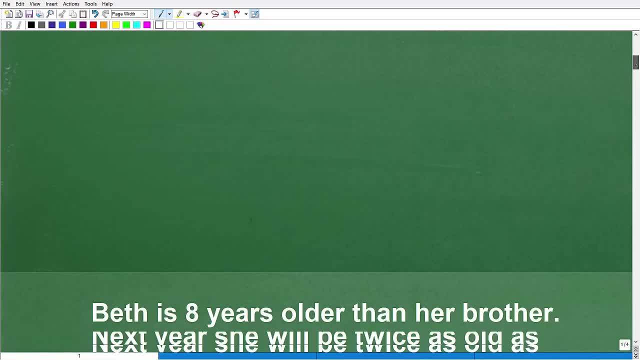 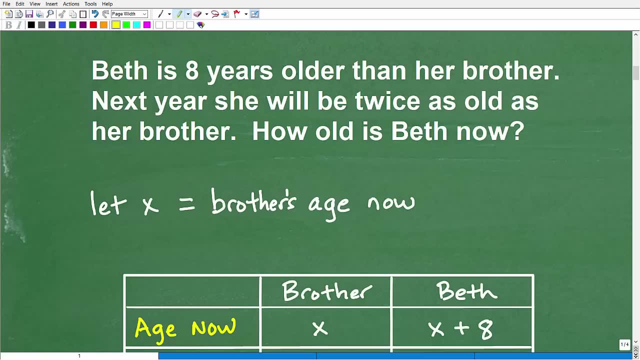 yourself to do this stuff on your own, okay, so let's get to the problem. all right? so obviously i kind of already did this in advance, and here we go: beth is eight years older than her brother, okay, so beth, all right, is currently eight years older. 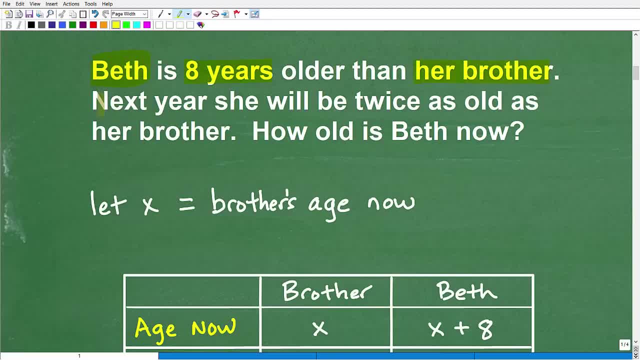 than her brother. so we got beth and her brother, okay, next year. next year she'll be twice as old as her brother. how old is beth now? okay, so we're talking about next year, all right. so let's go back here reread the problem: we got next year. we're not talking about next year, right? they want to. 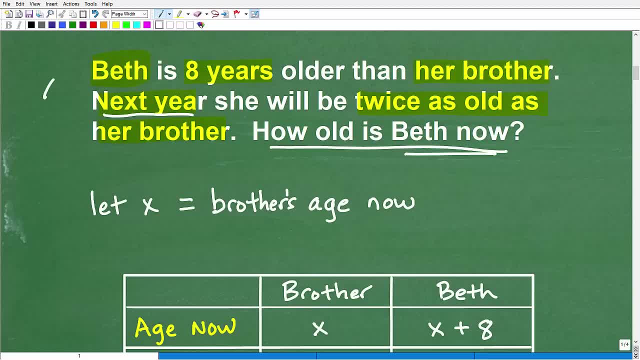 know how old is she right now? okay, so right now, beth is eight years older than her brother. okay, so beth is eight years older than her brother currently. okay, next year she's going to be twice as old as her brother, but remember how old is beth now. well, we need to focus in on her present. 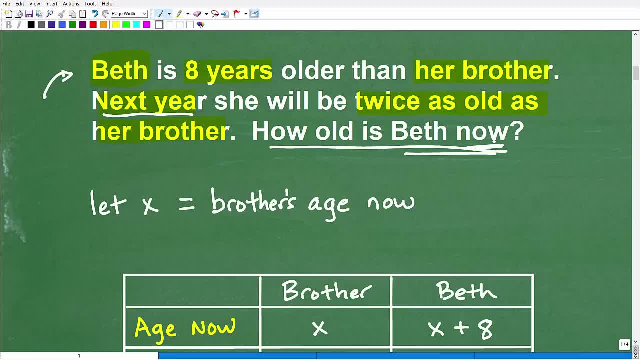 age, not her next year, next year's age. so here i'm going to go ahead and use the variable x, and this is where you would like to kind of play around with, uh, this type of problem. but we need to kind of get a baseline. so beth is eight years older than her brother. well, let's, let's. 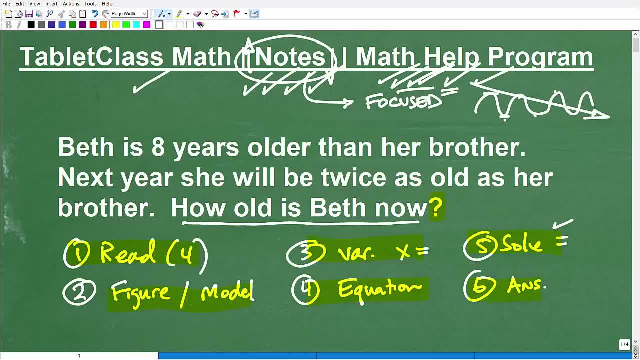 you're going to be like: oh, that was easy, remember, watching someone do math is not the same as learning math. okay, now i'm here to help you, obviously, but you should always try to challenge yourself to do this stuff on your own, okay, so let's get to the problem. all right, so obviously. 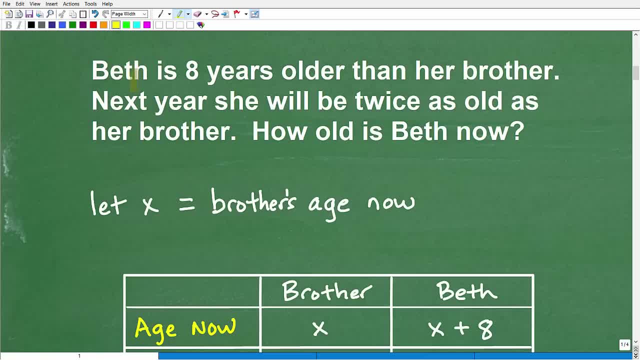 i kind of already did this in advance. and here we go. beth is eight years older than her brother, okay. so beth, all right, is currently eight years older than her brother. so we got beth and her brother, okay, next year. next year she'll be twice as old. 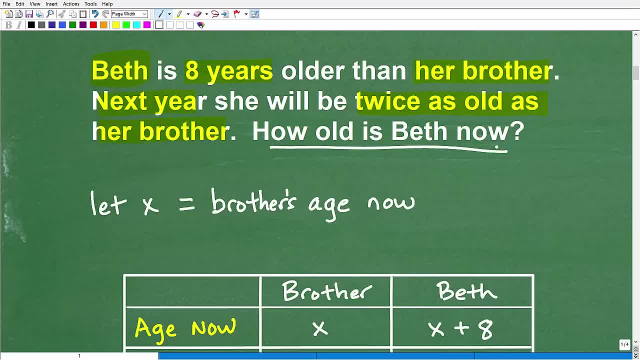 as her brother. how old is beth now? okay, so we're talking about next year, all right, so let's go back here reread the problem: we got next year, we're not talking about next year, right? they want to know how old is she right now? okay, so right now, beth is eight years older than her brother, okay, so 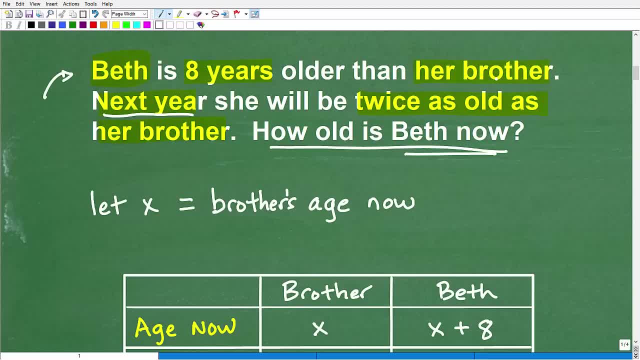 is eight years older than her brother currently. okay, next year she's going to be twice as older as her brother, but remember how old is beth now? well, we need to focus in on her present age and not her next year, next year's age. so here i'm going to go ahead and use the variable x and 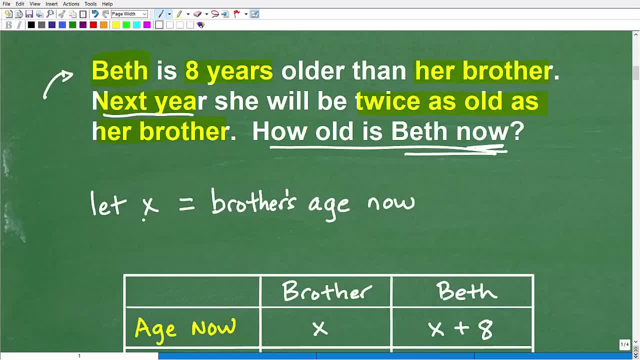 this is where you would like to kind of play around with, uh, this type of prom, but we need to kind of get a baseline. so beth is eight years older than her brother. well, let's, let's pick a variable. we don't know her brother's age. we don't know her age. let's just say her, uh, her brother is. 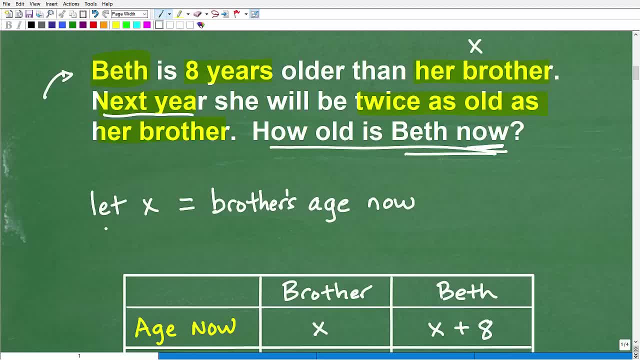 x years old right now. okay, so we're going to let x equal her brother's age currently right now. okay, so, with that being uh stated, we can determine. if i knew her brother's age right now. i know she's eight years older than whatever her brother's age, so if i get this x, i can definitely determine. 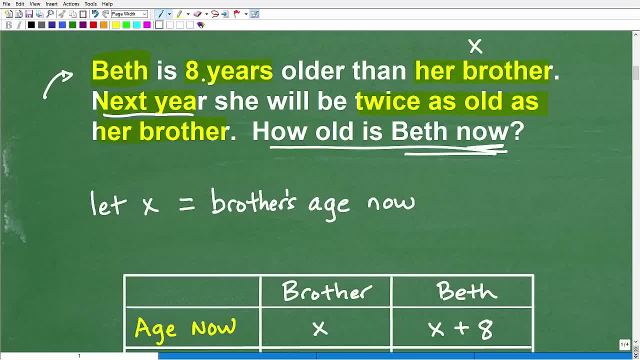 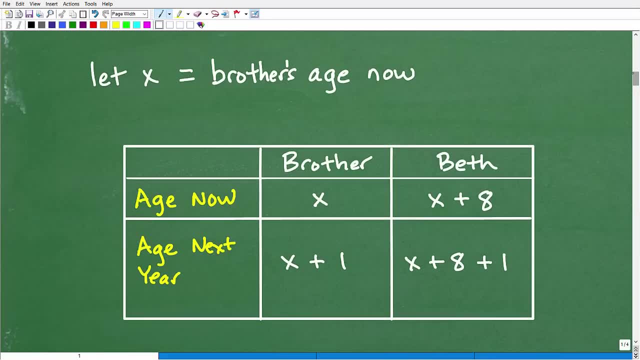 her current age. best, uh, current age, gotta just add eight years on to her brother's age. so, uh, now, when you're dealing with an age word problem or any kind of algebra problem, it's very, very useful to organize um the situation in a nice table. okay, so let's go ahead and take a look at this table. 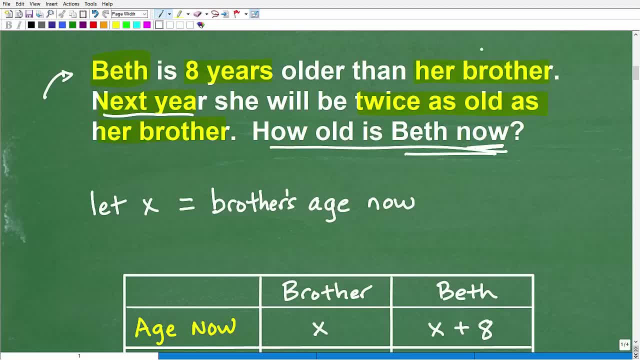 pick a variable. we don't know her brother's age, we don't know her age, let's just say her: uh, her brother is x years old right now. okay, so we're going to let x equal her brother's age currently right now. okay, so, with that being uh stated, we can determine if i knew her brother's age, right? 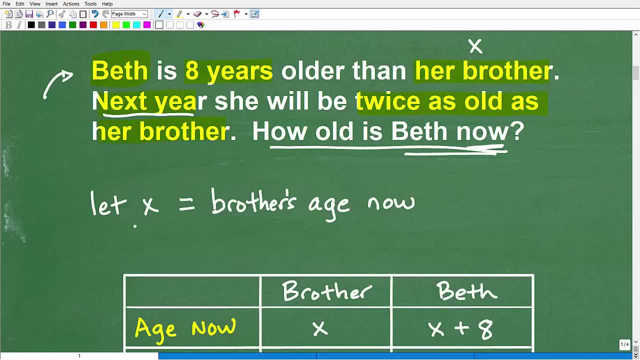 now i know she's eight years older than whatever her brother's age. so if i get this x, i can definitely determine her current age. beth's current age gotta just add eight years onto her brother's age. so, uh, now, when you're dealing with an age word problem or any kind of algebra, 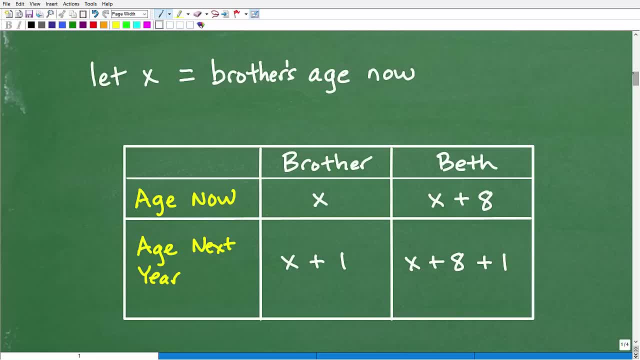 or problem. it's very, very useful to organize um the situation in a nice table. okay, so let's go ahead and take a look at this table. this is a very um classic kind of setup to solve these problems. so once you understand this kind of setup, you can use tables in algebra to solve. 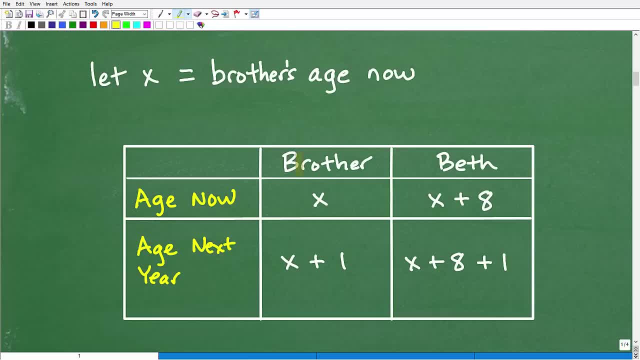 these word problems. so let's take a look at the information. we have her, uh, the brother, and we have beth. okay, so brother and her beth, and we have two kind of time frames: we have now their ages right now and then we have their ages next year. so, remember, we decided to let x equal to her brother's. 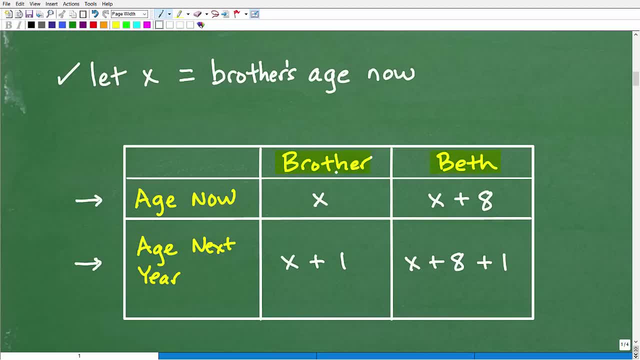 age right now. so let's go and fill out this table. so the brother's age right now is x, okay, and we know right now beth is eight years older than her brother. so whatever her brother's age is, it's x, right plus eight. that's beth's age right now. okay, so this is the current situation, so you got to. 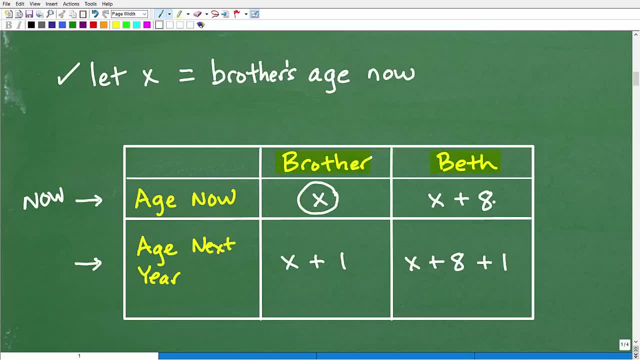 start someplace. we started with x and beth would be x plus eight. all right, now let's talk about next year. all right, so this is one year from now. okay, how old is her brother going to be? well, whatever his age is, we're going to add on one year. so their age next year, the brother's going to be x. 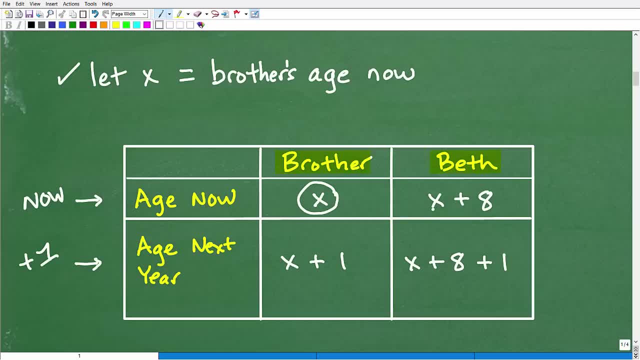 plus one, okay, and beth will be- uh, she's currently right now, so we're going to add on one year, so x plus eight. but next year she's going to be x plus eight plus one, okay, so both of them are going to be one year older. so, based upon this, we have some good algebra expressions for right now, okay. 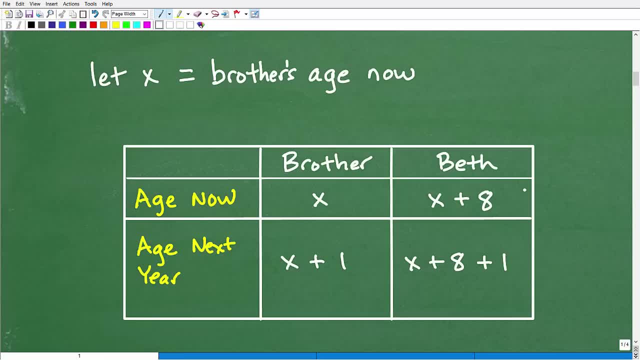 this is a very um classic kind of setup to solve these problems. so once you understand this kind of setup, you can use tables in algebra to solve these word problems. so let's take a look at the information. we have her, uh, the brother, and we have beth. okay, so, brother, 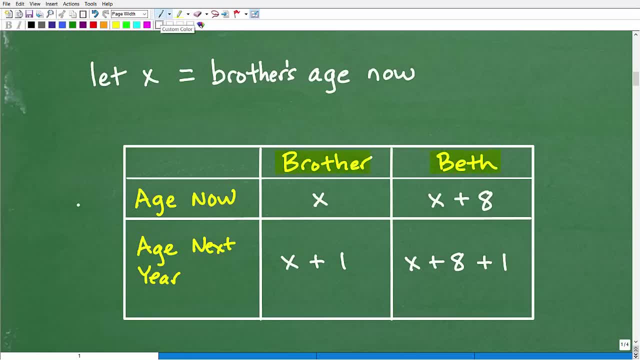 and her beth, and we have two kind of time frames. we have now their ages right now and then we have their ages next year. so, remember, we decided to let x equal to her brother's age right now. so let's go and fill out this table. so your, the brother's age right now is x, okay, and we know right now, beth. 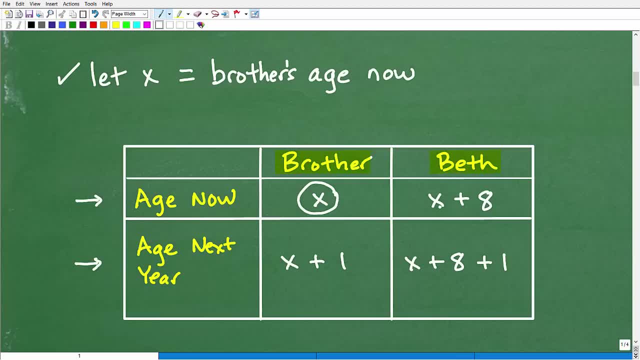 is eight years older than her brother, so whatever her brother's age is, it's x right plus eight. that's beth's age right now. okay, so this is the current situation. so you got to start someplace. we started with x and beth would be x plus eight. all right, now, let's talk about next year, all right, so this? 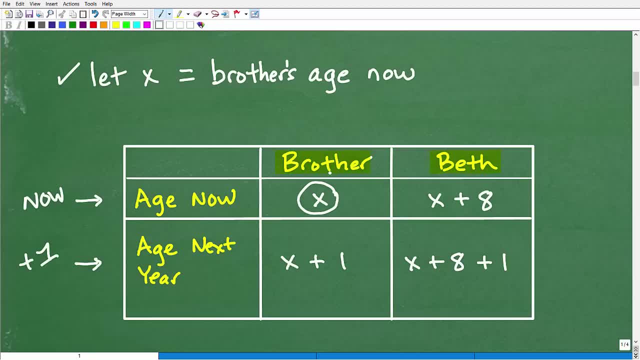 is one year from now. okay, how old is her brother going to be? well, whatever his age is, we're going to add on one year. so their age next year the brother is going to be x plus eight. so we're going to be x plus one, okay, and beth will be. uh, she's currently right now x plus eight, but next year. 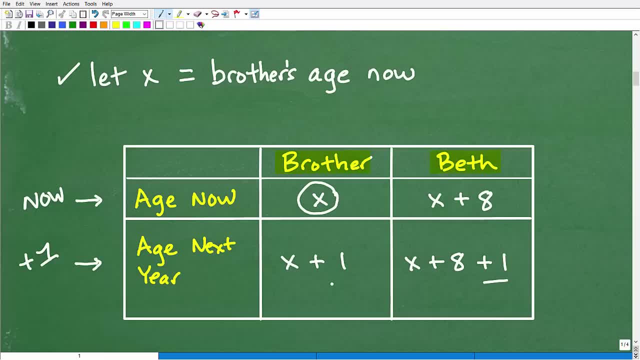 she's going to be x plus eight plus one, okay she's. both of them are going to be one year older. so, based upon this, we have some good algebra expressions for um right now. okay, their situation right now, their age is right now and their age is next year. and we have these all in terms of our 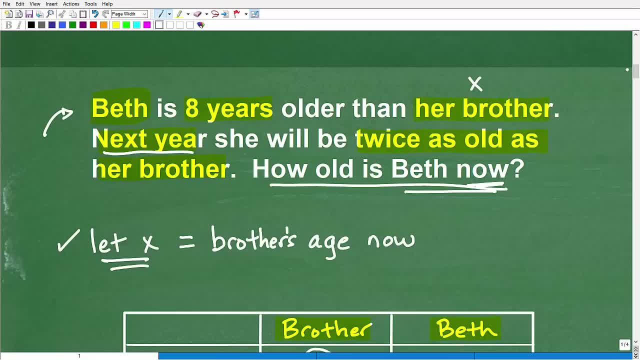 variable x. okay, all right, so now we can go back and reread the problem. remember, you know these things that i'm telling you. uh, you know i'm not making this up, you know, when i see like read the problem, read the problem, read the problem, that's what i mean: reread the problem, all right. so now, uh, let's go. 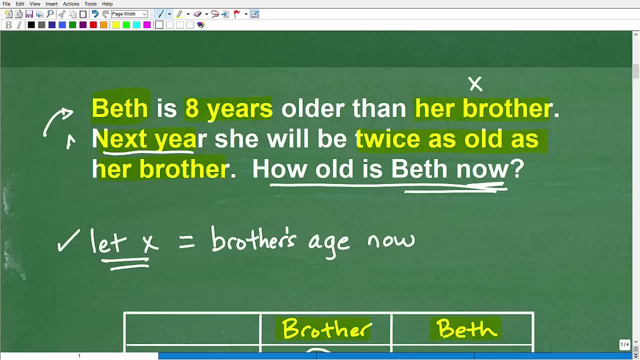 back and reread this part next year. we're going to need this part right here. we need to build an equation. is what i'm getting at? all, right, we need to build an equation. we have a nice table, but we need some sort of relationship. so right in this part of the problem, he says next year she will be. 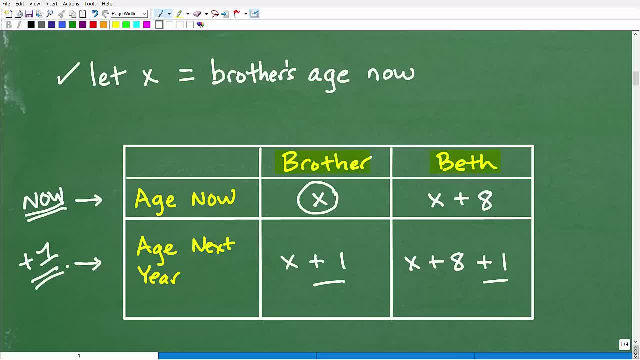 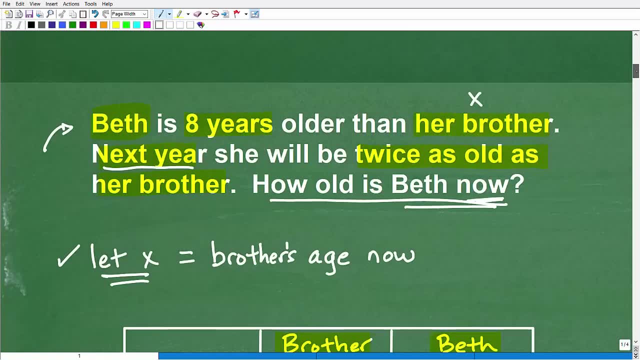 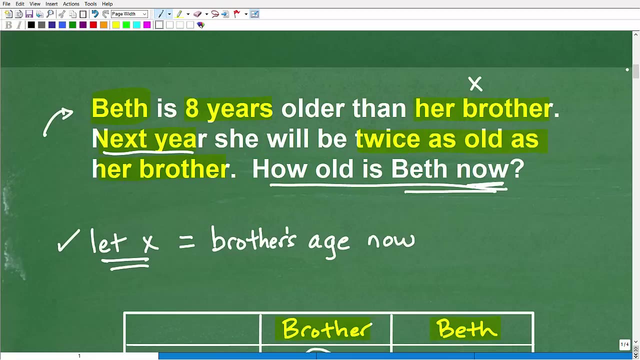 their situation right now, their ages right now and their ages next year, and we have these all in terms of our variable x. okay, all right, so now we can go back and reread the problem. remember, you know these things that i'm telling you. uh, you know i'm not making this up. you know, when i say like read the problem, read the problem read. 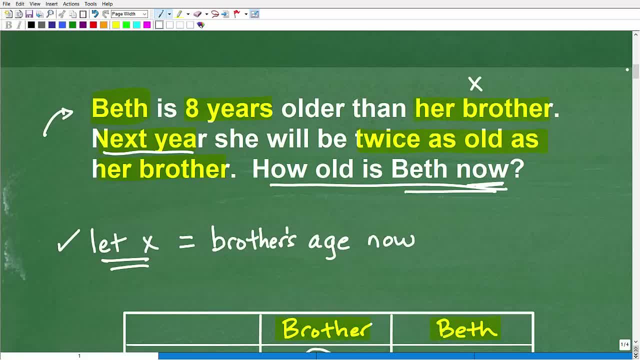 the problem. that's what i mean. reread the problem, all right. so now, uh, let's go back and reread this part. next year we're going to need this part right here. we need to build an equation. is what i'm getting at. all right, we need to build an equation. we have a nice table, but we need some sort of 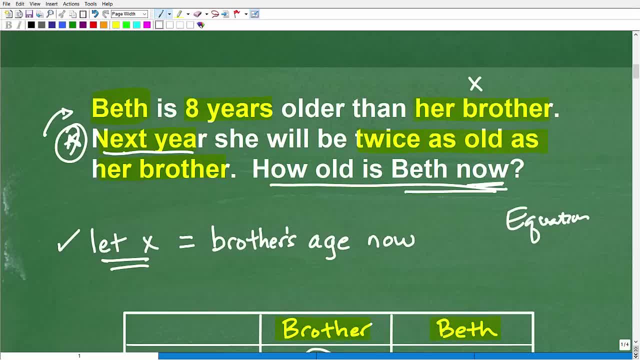 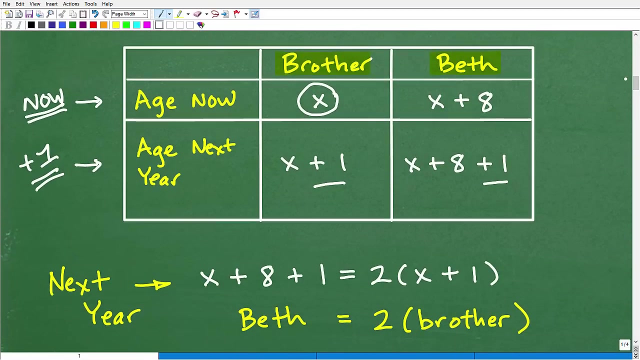 relationship. so, right in this part of the problem, he says: next year she will be twice as old as her brother. so we got to bring this part of the problem and this, this fact, to help us solve, uh, to help us establish an equation. so next year she will be twice as old as her brother, so we can use this table here to build an equation. so next, 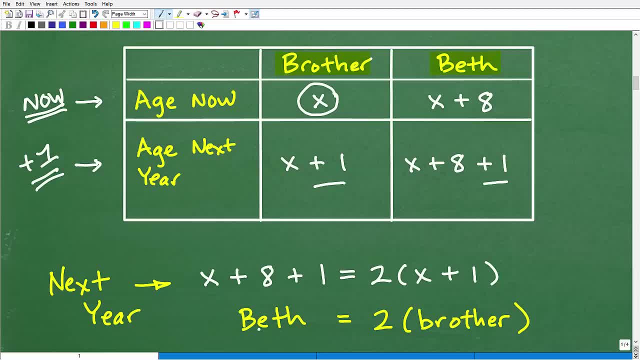 year beth. okay, so here's beth right here. uh, so her, her, her age next year is going to be what? x plus a plus one. we already determined that, okay. so this is beth next year age, and her brother's age next year is going to be x plus one. okay, but she is going to be whatever. 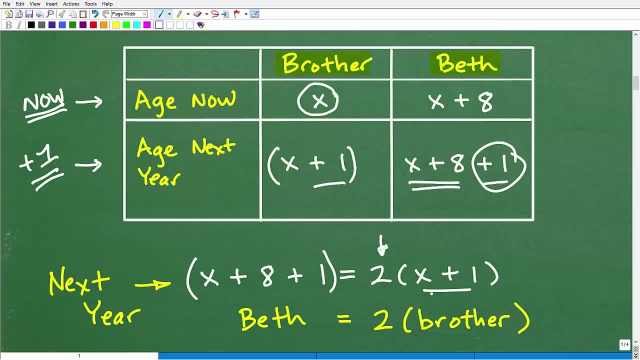 her age is it's going to be twice her brother's age. so next year her brother will be x plus one, okay, so, whatever his age, we multiply by two. okay, that's what her age is going to be next year. so really make sure you understand this uh relationship. okay, so next year beth is going to be. 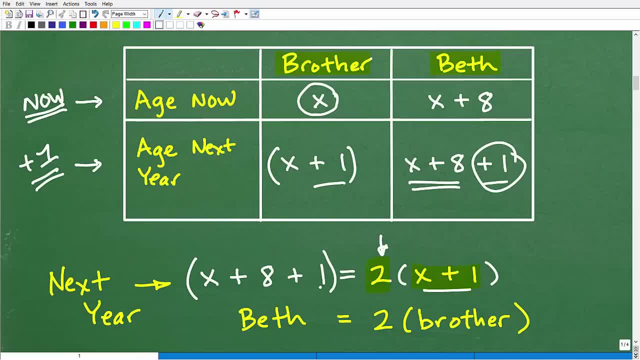 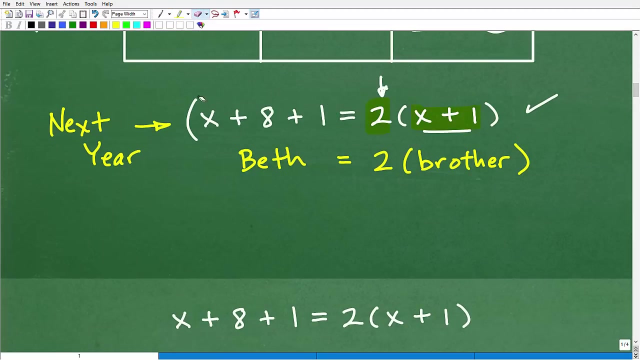 um, x plus eight plus one, but she's also going to be twice her brother's age, so we can set up this equation. this is very, very important and this is, uh, you know, pretty, you know, hopefully easier to determine once we have our nice table here. okay, all right, so now we have to solve for x. we finally got ourselves a nice. 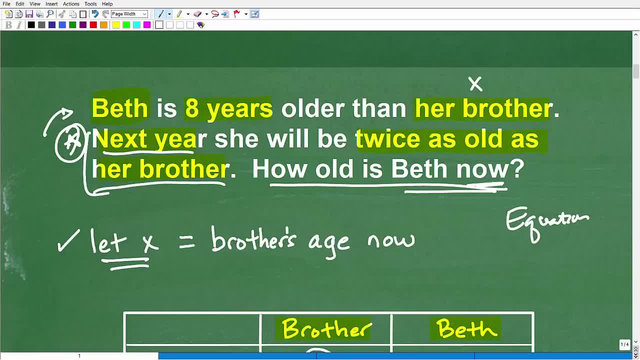 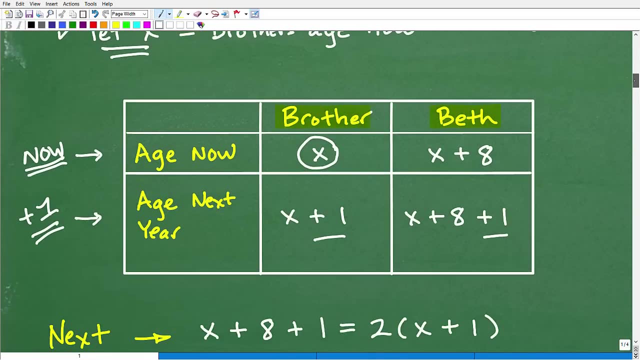 twice as old as her brother. so we got to bring this part of the problem and this, this fact to help us solve, uh, to help us establish an equation. so next year she will be twice as old as her brother, so we can use this table here to build an equation. so next year, beth. okay, so here's beth. 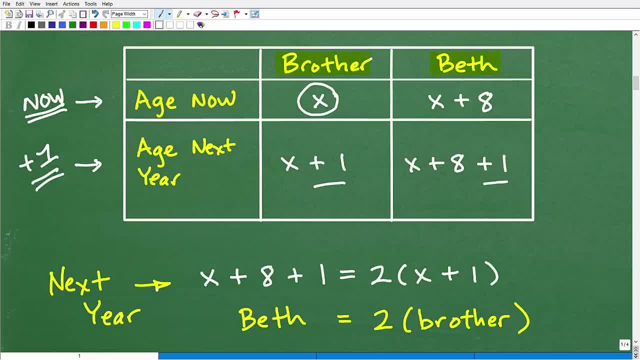 right here. uh, so her, her, her age next year is going to be what plus one? we already determined that. okay, so this is beth next year, her age and her brother's age next year is going to be x plus one. okay, but she is going to be whatever her age is. it's going to. 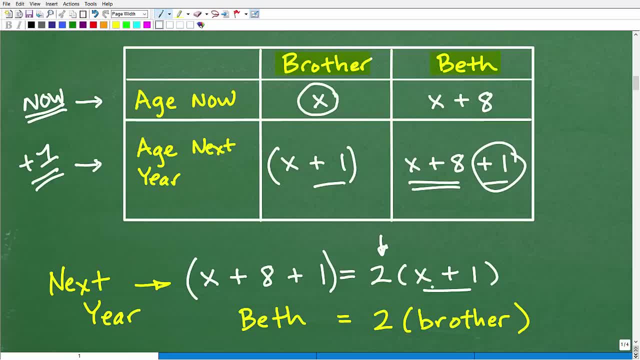 be twice her brother's age. so next year her brother will be x plus one. okay, so, whatever his age, we multiply by two. okay, that's what her age is going to be next year. so really make sure you understand this uh relationship. okay, so next year beth is going to be um x plus eight plus one, but she's also going to be twice her. 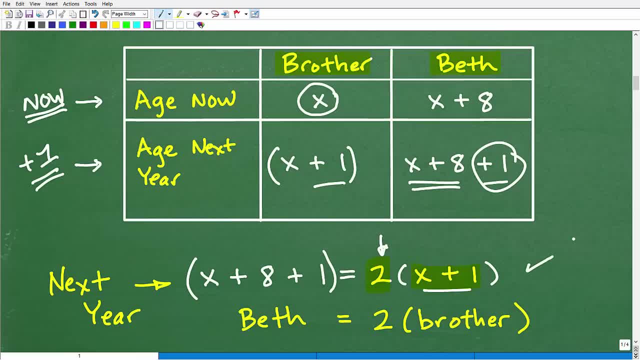 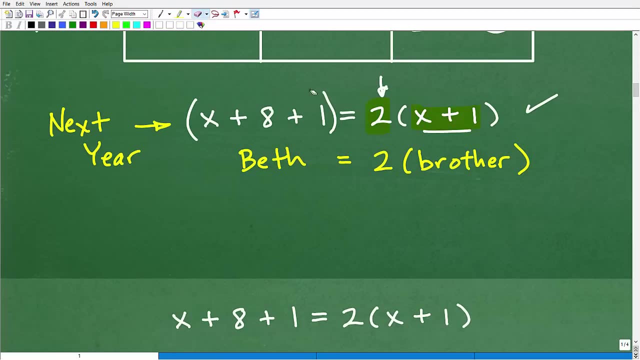 brother's age so we can set up this equation. this is very, very important and this is, uh, you know, pretty, you know, hopefully easier to determine once we have our nice table here. okay, all right, so now we have to solve for x. we finally got ourselves a nice equation involving 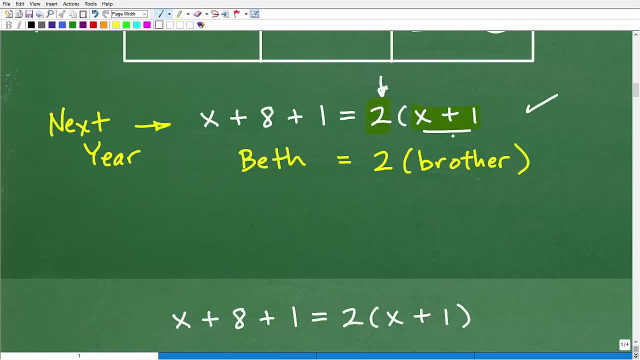 x. and now this requires your ability to solve basic equations. again, when i talked about word prompts, you need to have skills. okay, then we apply those skills in an application to solve a word prompt. so oftentimes you're not gonna be able to solve a word problem if you don't have the basic skills that you're studying. so the step, you know what? 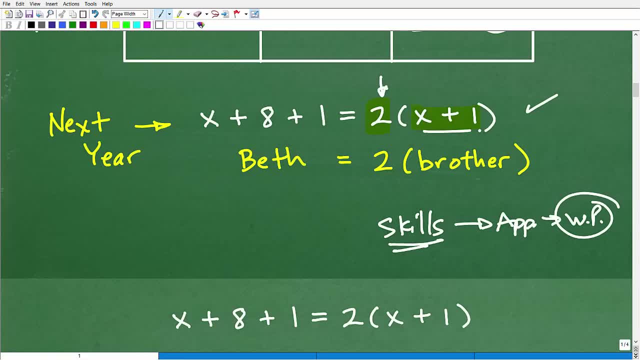 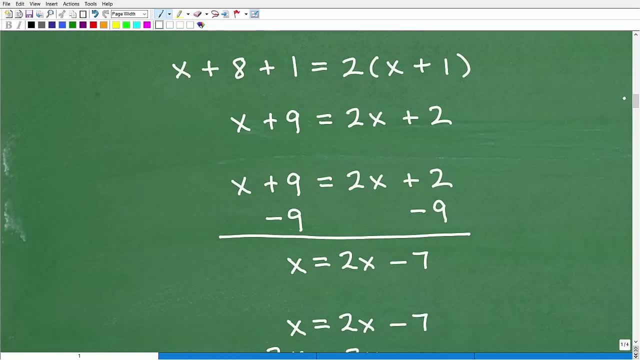 you're studying right here is, um, you know how to solve a linear equations. okay, that's uh, generally you know the kind of the topic algebra skills if you're well solving equations, so at this point hopefully most of you can solve this equation. now, if you, if you can't solve this equation, then you're really really going to be struggling with the 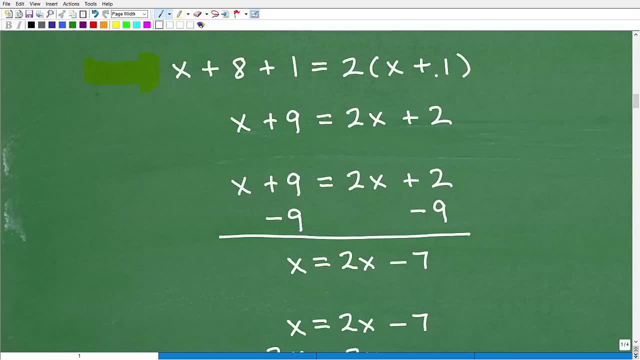 word problem? uh, like this. so what do you do if you, if you're struggling solving this equation, well, you're going to have to go back and review how to solve linear equations. okay, don't continue to struggle with the word problem. it's not going to make any sense. 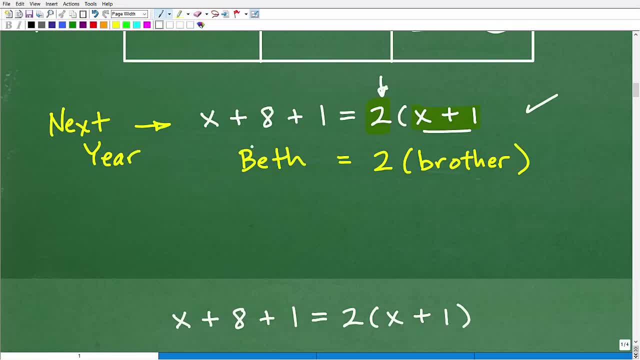 equation involving x. and now this requires your ability to solve basic equations again. um, when i talked about word problems, you need to have skills. okay, then we apply those skills in an application to solve a word prompt, so oftentimes you're not going to be able to solve. 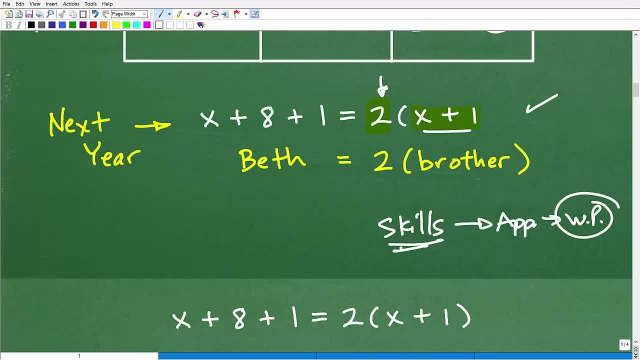 a word problem if you don't have the basic skills that you're studying. so the step you know what you're studying right here is: um, you know how to solve linear equations? okay, that's generally. you know the kind of the topic algebra skills if you will solving equations. so at this point, 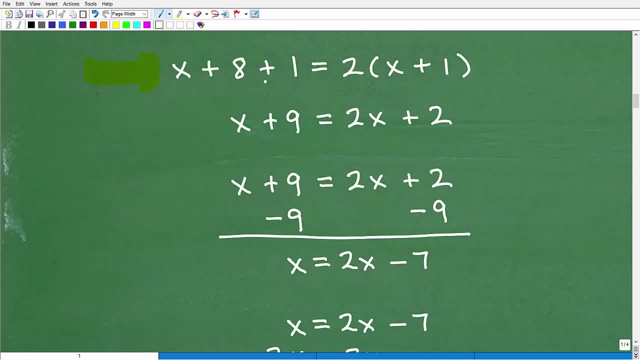 hopefully most of you can solve the algebra skills and then you can solve the linear equations. now, if you, if you can't solve this equation, then you're really, really going to be struggling with the word problem like this. so what do you do if you, if you're struggling solving this equation? 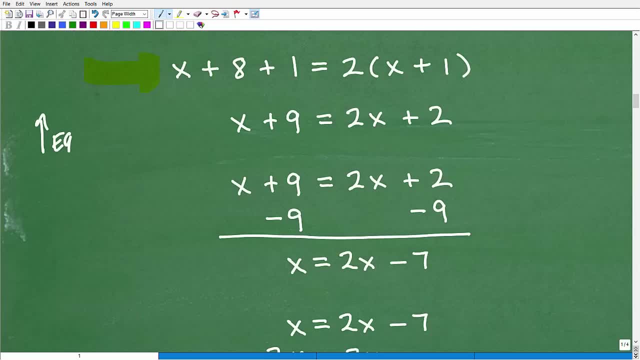 well, you're going to have to go back and review how to solve linear equations. okay, don't continue to struggle with the word problem. it's not going to make any sense because you need to up your skills with equations. so go back and review, strengthen and then come back to this problem. 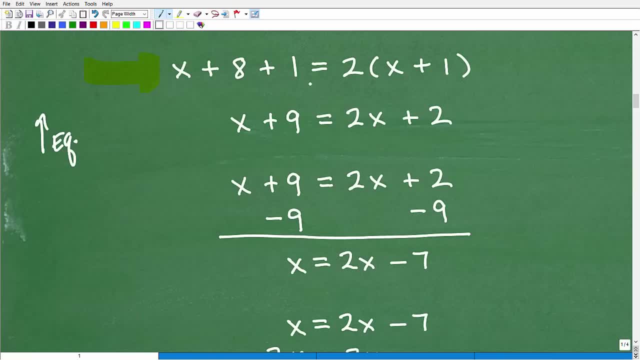 but let's go ahead and walk through the equation. so we have x plus eight plus one. one is equal to two x uh, or equal to two times x plus one. so, uh, we got x plus eight plus one. that's going to be the same as x plus nine. and then here i can use a distributive property: okay, so two times. 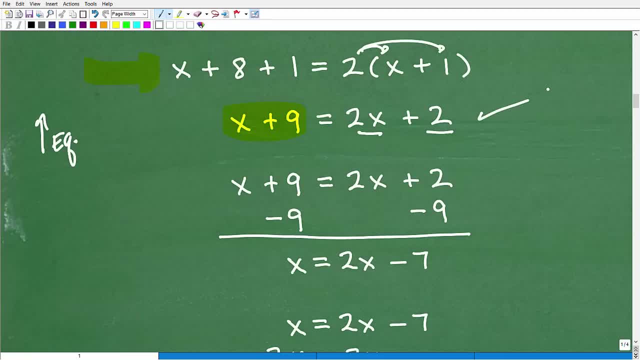 x is two x, and two times one is two. okay, so that's where we're at, and now let's go ahead. and we don't have any alike terms on either side of the equations, remember when we're solving numbers on the right? so i'm going to start moving over. uh, the number here i have on the left hand. 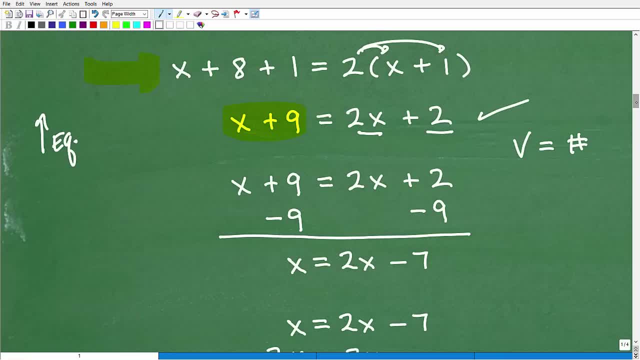 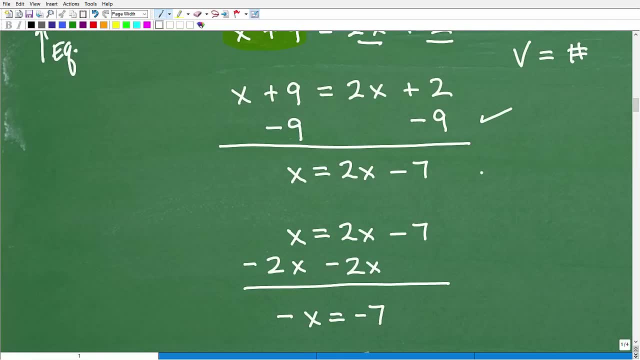 side, that's nine. so i'm going to subtract nine from both sides of the equation. that's what i'm doing right here. so i get: x is equal to two x minus seven. so be careful with your positive negative numbers. now notice how i'm showing you all the work. okay, do you think you want to be? 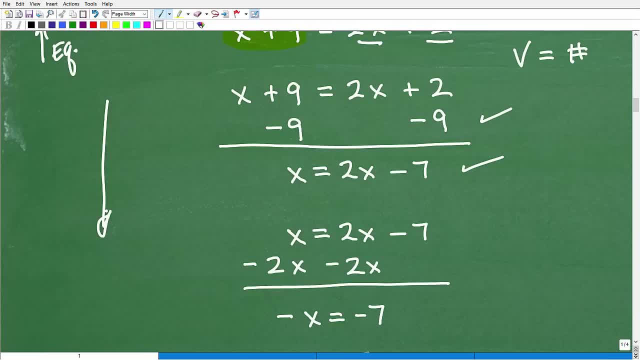 doing the same thing when you turn in your uh test or quiz or your homework. yes, yes, yes, okay, do not do your homework in a sloppy manner. don't be like, because what you're doing is it's uh. you're practicing bad habits, right? so, my you? 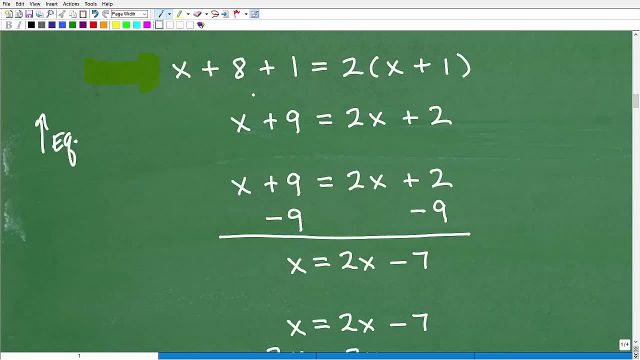 because you need to up your skills with equations. so go back and review, strengthen and then come back to this problem. but let's go ahead and walk through the equation. so we have x plus 8 plus 1 is equal to 2x, or equal to 2 times x plus 1.. so we have x plus 8 plus 1. that's going to be the same. 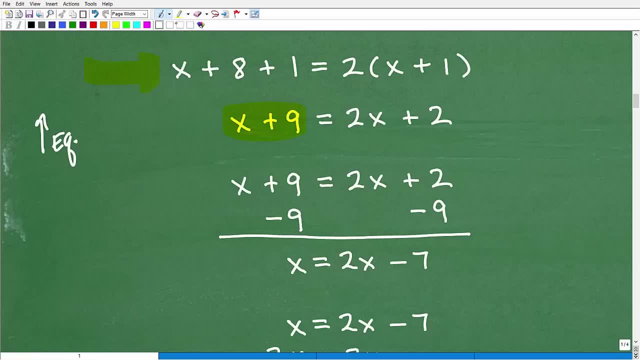 as x plus 9.. and then here i can use the distributive property. okay, so 2 times x is 2x and 2 times 1 is 2.. okay, so that's where we're at, and now let's go ahead. and um, we don't have any. 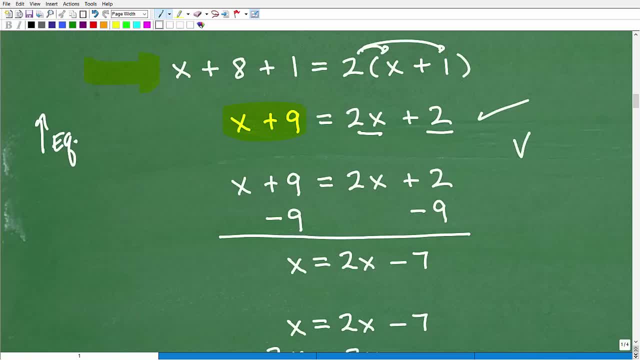 other numbers on either side of the equations. remember, when we're solving equations we want the variables on the left and the numbers on the right. so i'm going to start moving over. uh, the number here i have on the left-hand side, that's 9.. so i'm going to subtract 9 from both sides of the. 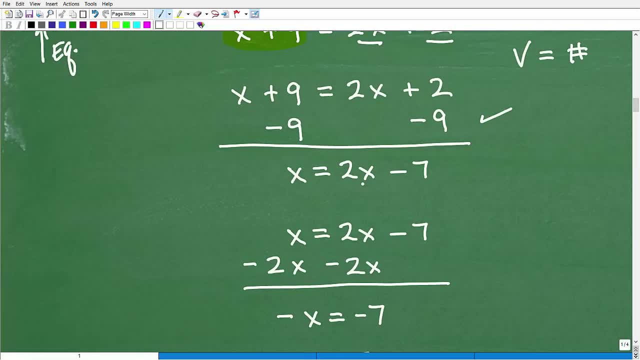 equation. that's what i'm doing right here. so i get: x is equal to 2x minus 7.. so be careful with your positive negative numbers. now notice how i'm showing you all the work, okay. do you think you want to be doing the same thing when you're turning your uh test or quiz, or your homework? 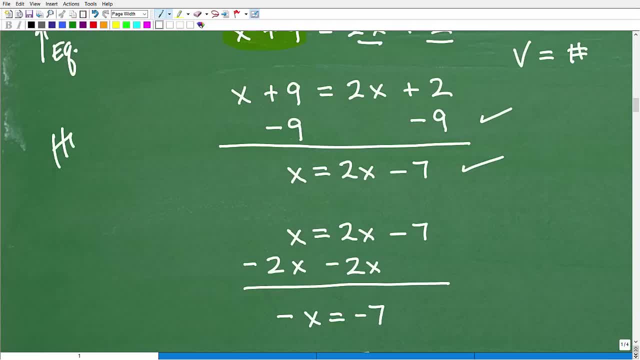 yes, yes, yes, okay, do not do your homework in a sloppy manner. don't be like, because what you're doing is it's uh, you're practicing bad habits, right? so my you know, philosophy is: i'd rather you not do math at all. if you're not going to do math the right way, don't do it at all, because if 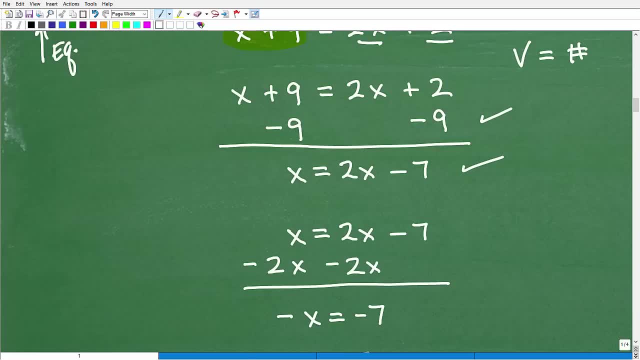 you're going to practice it in a poor manner, then all you're doing is instilling bad habits. okay, you want to be neat, clear and structured? show your work one step at a time. okay, so now we have: x equals 2x minus 7. i got to move that 7 over to the other side. uh, i'm sorry, um, excuse me, not the 7. 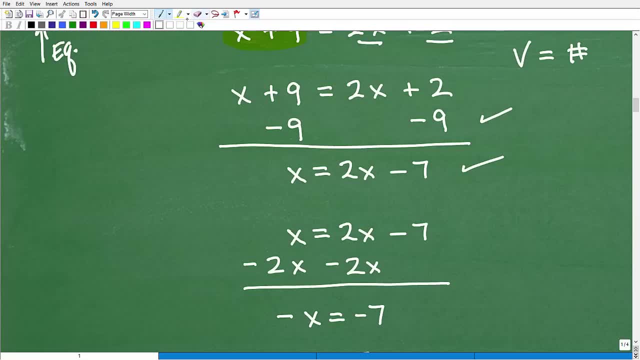 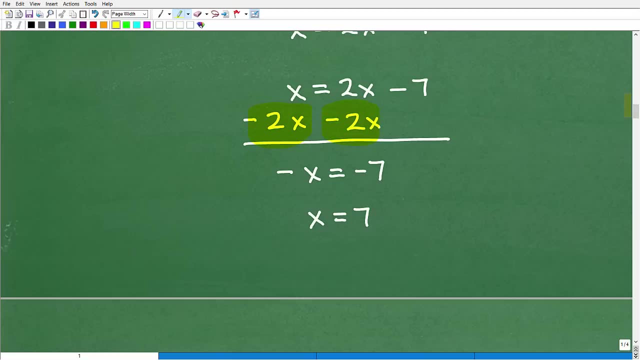 over the 7 is perfectly fine. i move the x over, so i'm subtracting now. uh, negative 2x from the other side. now, if you're again not quite understanding what i'm doing here, then you got to go back and watch my videos on solving equations in my algebra playlist. okay, so we end. 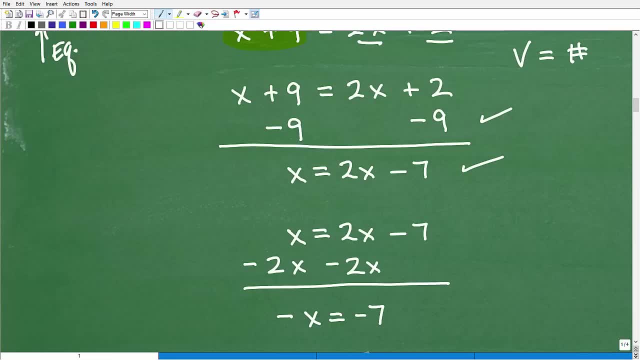 know philosophy is, i'd rather you not do math at all. if you're not going to do math the right way, don't do it at all, because if you're going to practice it in a poor manner, then all you're doing is instilling bad habits. okay, you want to be neat, clear and structured? show your work. 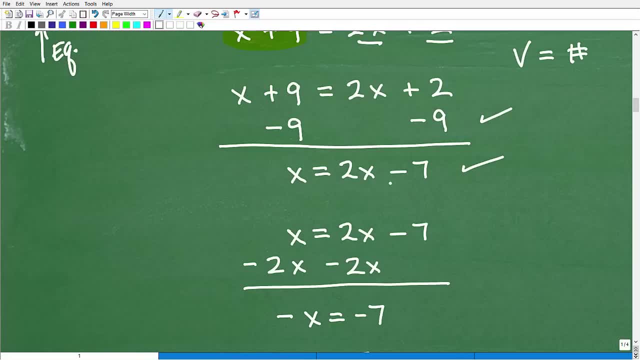 one step at a time. okay, so now we have x equals two x minus seven. i got to move that seven over to the other side. uh, i'm sorry, um, excuse me, not the seven over the seven's. perfectly fine, i gotta move the x over, so i'm subtracting now. uh, negative two x from the other side. now, if you're again not quite, 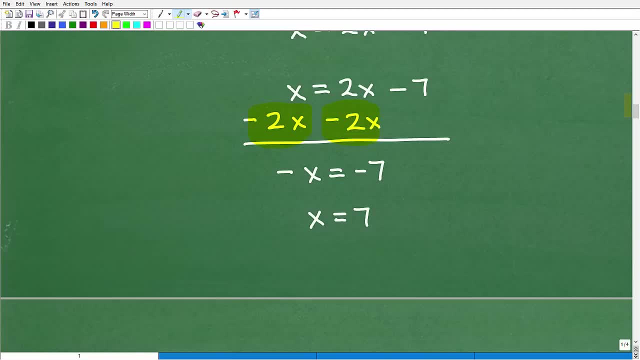 understanding what i'm doing here. then you got to go back and watch my videos on solving equations in my algebra playlist. okay, so we end up with negative x is equal to negative seven and that is equivalent to x is equal to seven. so at this point a lot of you would be so excited you'd be. 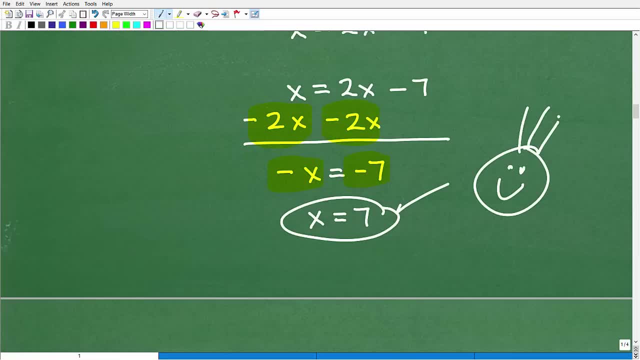 like i am so awesome in math. look at me, here you go, mr teacher. x is equal to seven. uh, you know, i need my a plus. can you please give my a plus? and then i turn around and give you a b, and then you're like, you know, you're like, you're like this, you know, you're like: hey, what's going on here? well, this is. 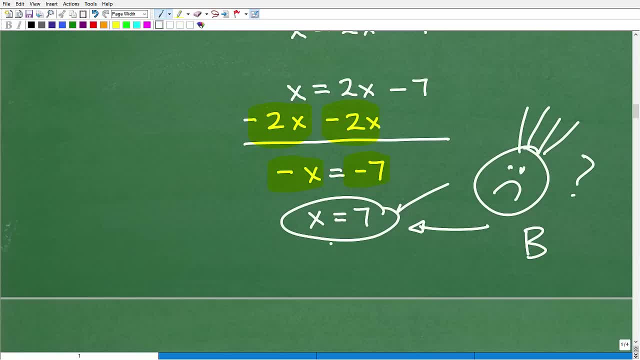 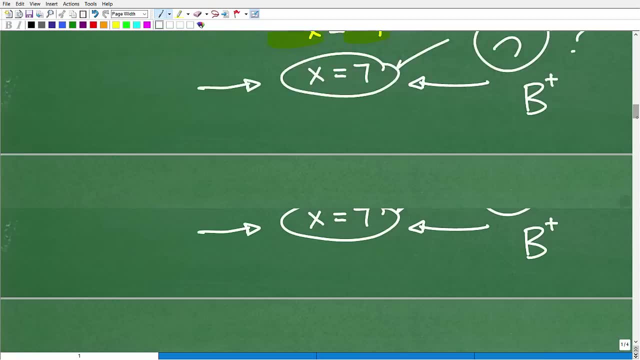 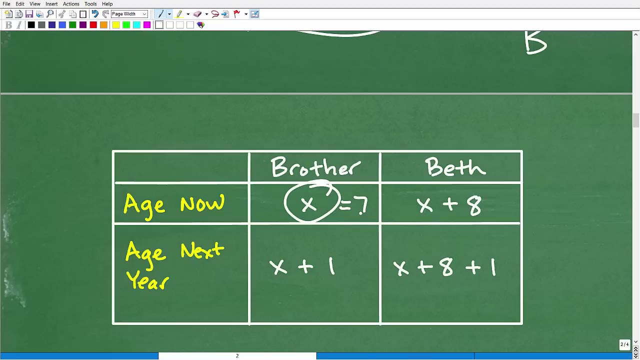 not answering the question. okay, i know you're excited and whatnot and you know, maybe i would give you a b plus i'd be. listen, listen, what is x equal to? well, remember x was equals to the brother's age. now, okay, so the brother is seven, but the question: remember what was the question? 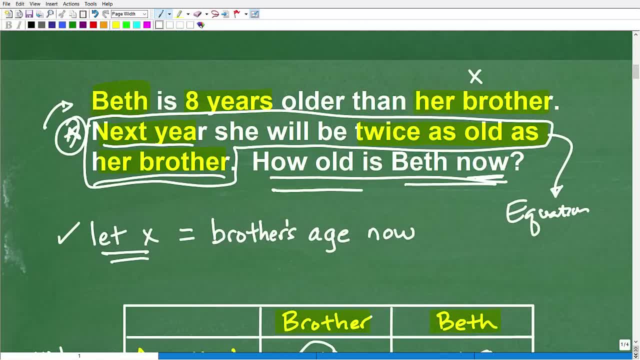 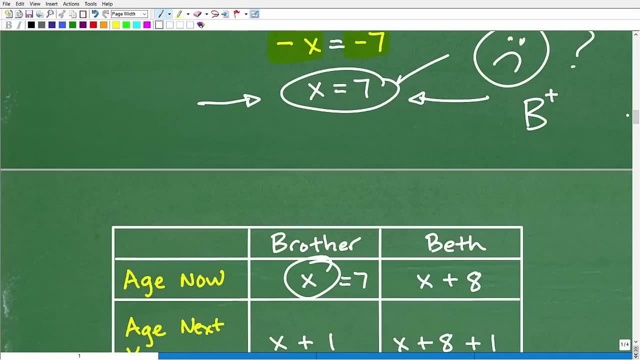 all right, let's go all the way up. the question is: how old is beth now? that's what the question's asking, not the brother's age. we need the brother's age, but the question is: how old is beth now? okay, so remember. everything i'm telling you comes from long years of experience teaching. okay. 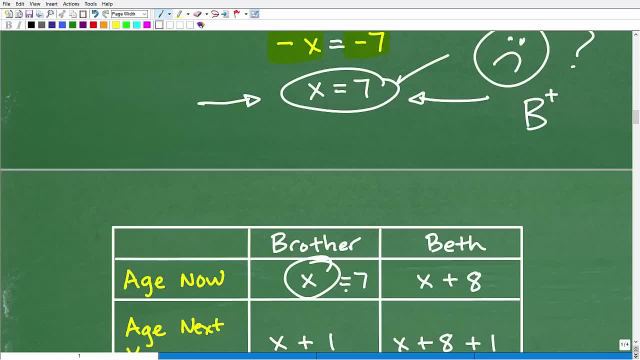 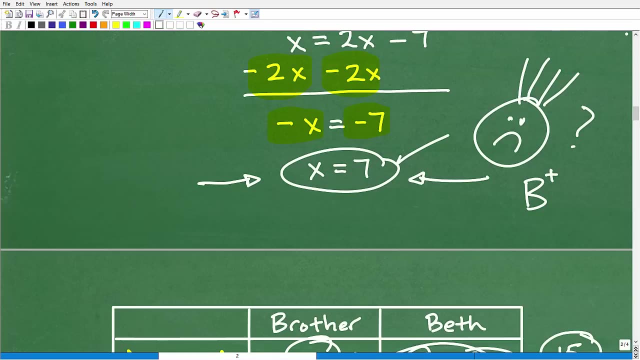 so how old is beth? now? well, i know her, her the brother is seven, so seven plus eight, okay, if that's, uh, uh, the brother's age. currently beth is 15 years old, okay, so you know, small little details are. are the difference between a, b and an a, all right. or a, d and an f? okay, math is made up with all these little things. 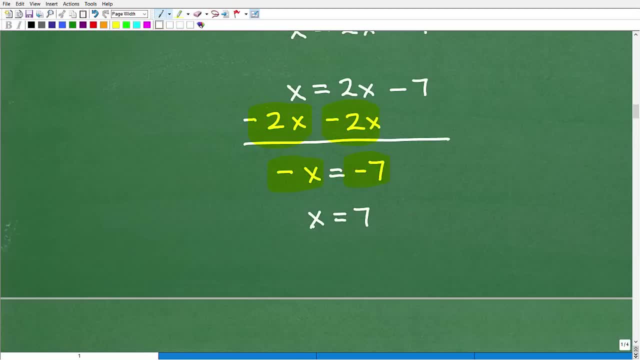 up with negative. x is equal to negative 7 and that is equivalent to x is equal to seven. so at this point a lot of you would be so excited you'd be like: i am so awesome in math. look at me, here you go, mr teacher. x is equal to seven. 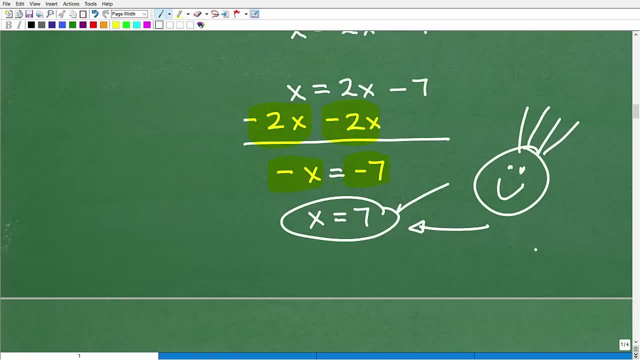 uh, you know, i need my a plus. can you please give my a plus? and then i turn around and give you a b and then you're like, you know, you're like, you're like this, you know, you're like, hey, what's going on here? well, this is not answering the question. okay, i know you're excited and whatnot, i know. 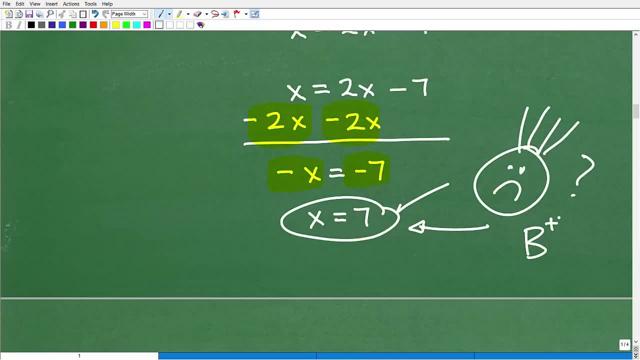 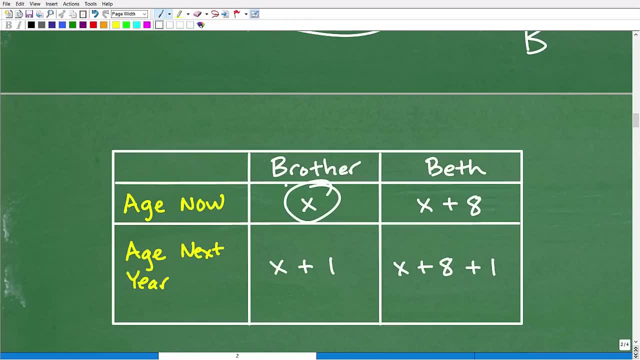 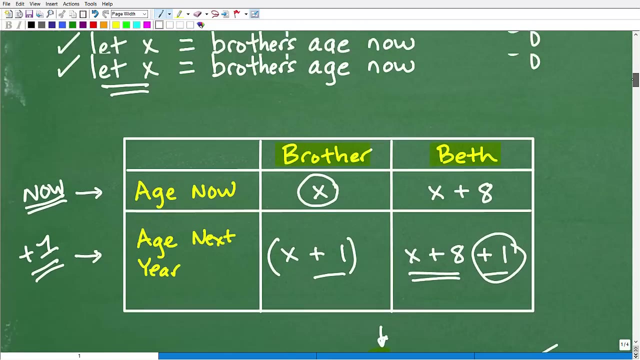 you know, maybe i would give you a b plus. i'd be like, listen, listen, what is x equal to? well, remember, x was equals to the brother's age. now, okay, so the brother is seven. but the question? remember what was the question? let's go all the way up. the question is: how old is beth? now, that's what the 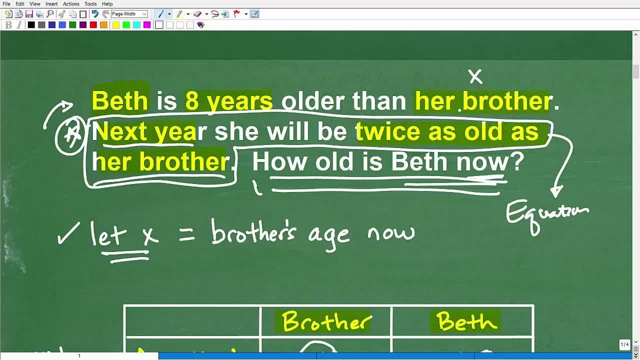 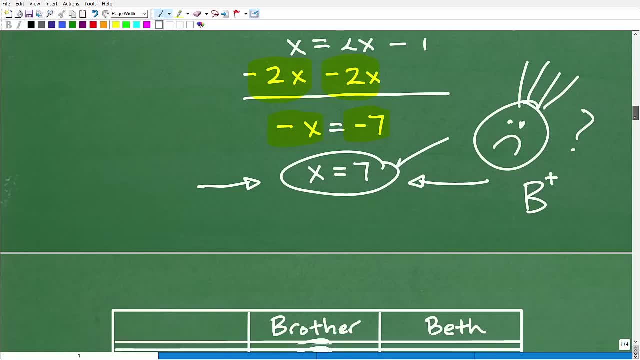 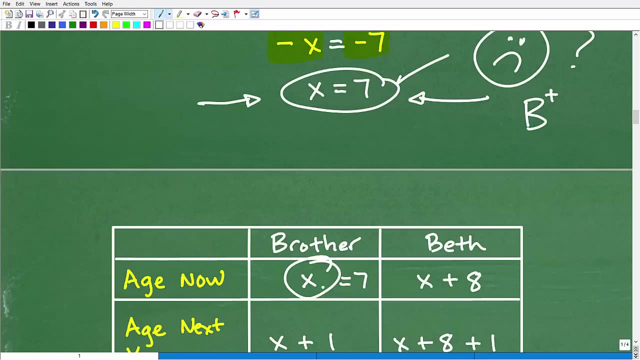 question's asking not the brother's age. we need the brother's age, but the question is how old is? so remember everything i'm telling you comes from long years of experience teaching. okay, so how old is beth now? well, i know her. the brother is seven, so seven plus eight. 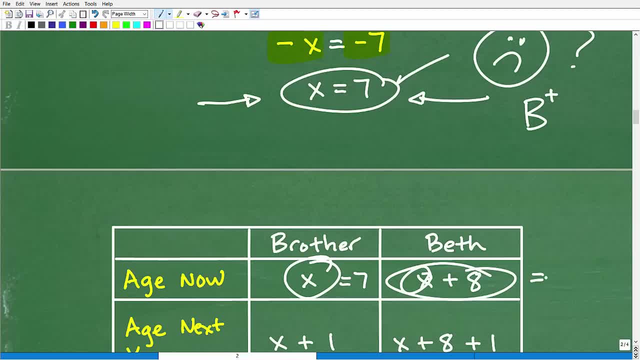 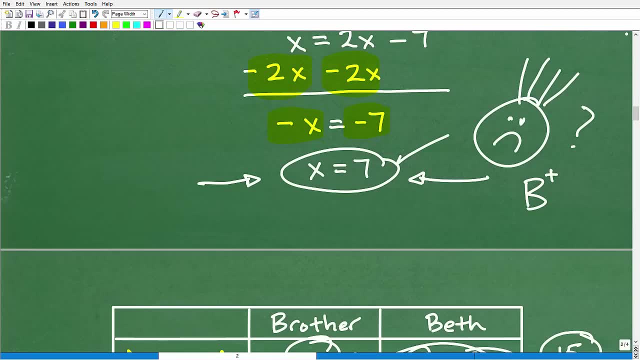 okay, if that's. uh. uh, the brother's age currently, beth is 15 years old, okay, so you know, small little details are. are the difference between a b and an a, all right. or a d and an f? okay. math is made up with all these little things, okay, and the worst thing to that. 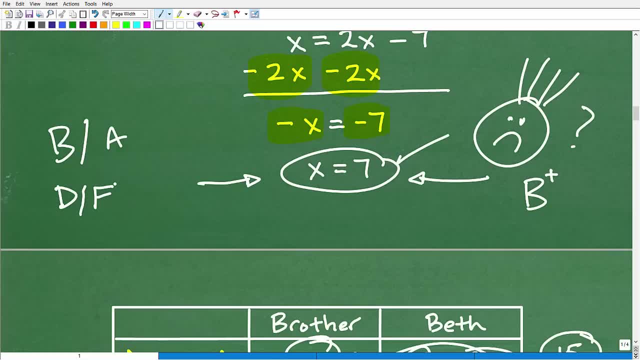 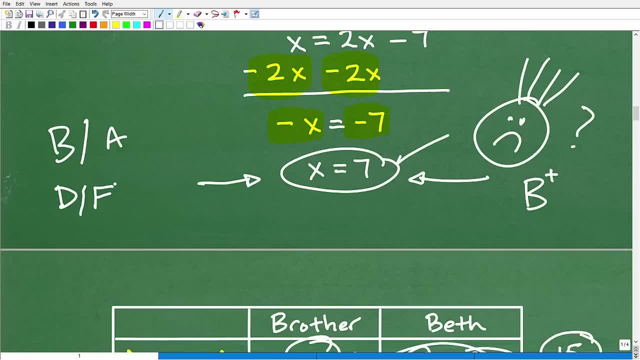 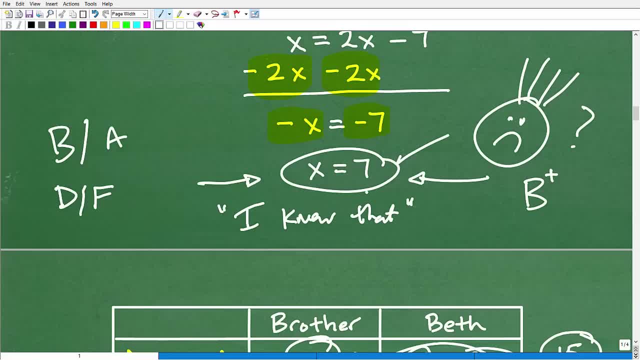 math. i knew that. i knew that, mr teacher, listen, yeah, i know i gave you x equals seven, but i knew that she was 15. listen, you know you don't want to be like this sad person. if you knew that, you got to like, do that okay. and why would that happen? well, someone could. someone could give you the. 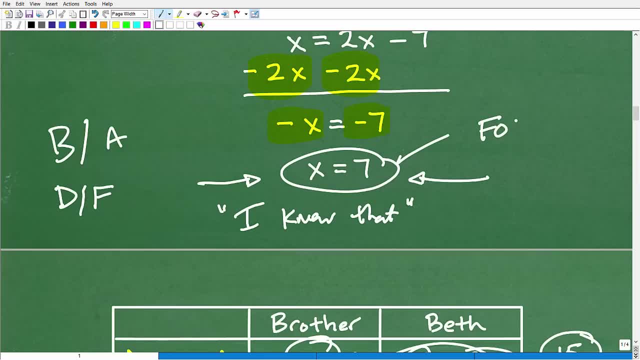 the wrong answer, because they're not remaining focused. math is a game of focus, okay, commitment, dedication, all right, and that's why a lot of people, i think, struggle with it, because they're just like, yeah, you know, i kind of like learn it, not learn it, not learn it, you know, or whatever. you can't learn math that way. 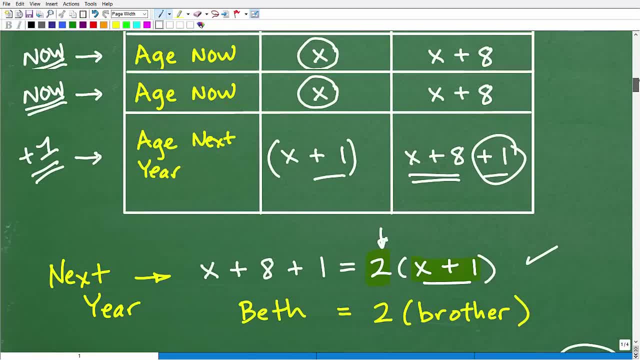 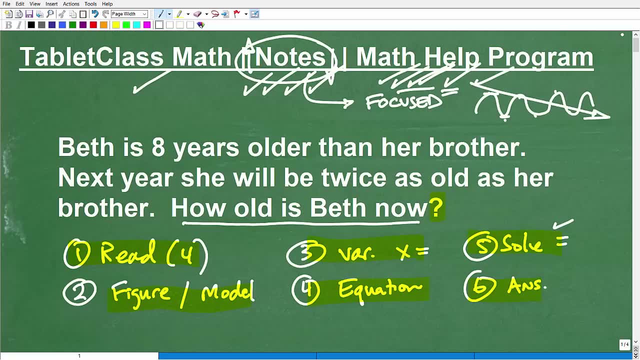 so if you're struggling in math, you got to really you know, um, you know, be honest with yourself, but i'm here to tell you absolutely, you can be a great at math. everyone could be, everyone could do excellent in mathematics. of course, we all have our own natural you know aptitudes and and whatnot, and some of you are are. 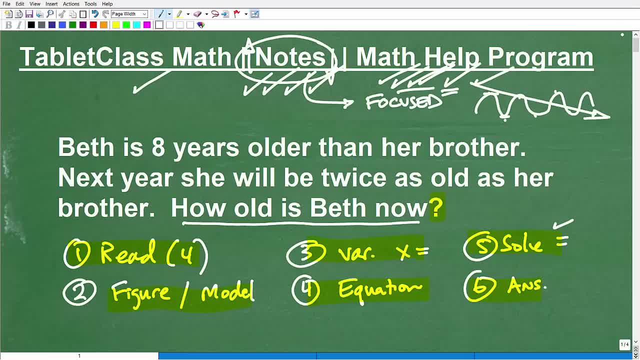 going to go much further in math than others. but for this level of math i tell you, it's been my experience- that almost you know, almost i mean, i mean- and i'm not trying to be, you know, exaggerate here- just about everyone can do very, very, very well in math. so if you're struggling in math then 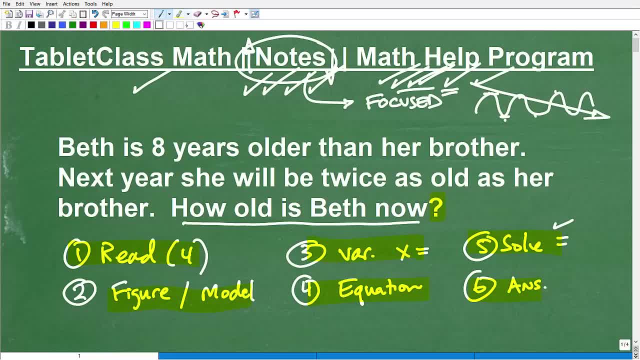 you know you're going to have to change your, change up your situation. okay, one, take a look at your notes. two, find a teacher that you're going to be able to teach you how to do it and you're going to like and understand. so if you're teaching, you're not connected with the teacher and you like my 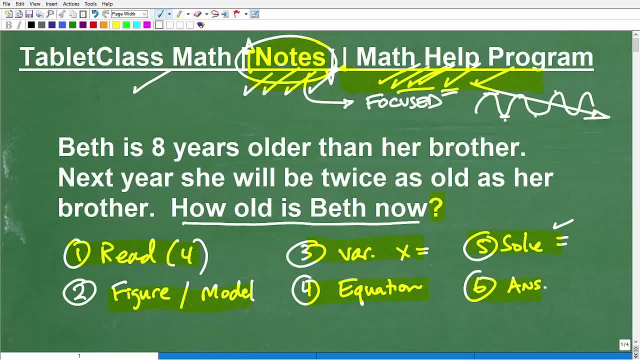 teaching. you know style, then you know, you know where to go to get help, all right. so if you like this video, if this really cleared up, uh, some stuff for you and helped you out with word problems, please consider smashing that like button. that would help me out. and please consider, uh, subscribing.